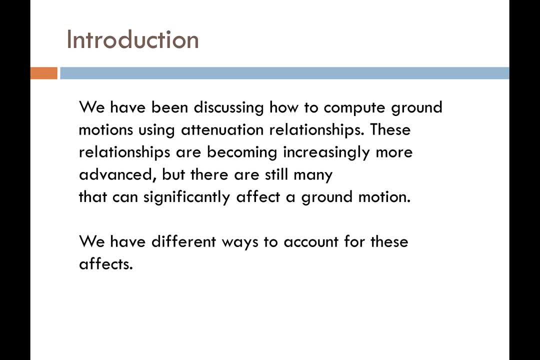 So that's a deterministic analysis, And you've even dipped your toes into the computation of probabilistic analyses, And so those are lots of fun, to say the least, And so what I want to talk about today, though, is understanding a little bit more about some factors that can affect ground motions on a local site level. 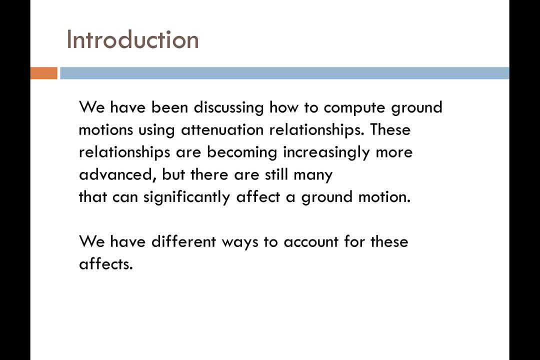 There's still a lot of things at the local site that can affect the intensity of the ground motions that are experienced, And a lot of these things can't really adequately or effectively be captured inside of just the attenuation relationships themselves, And so we're going to just walk through a few of those today. That's my goal. 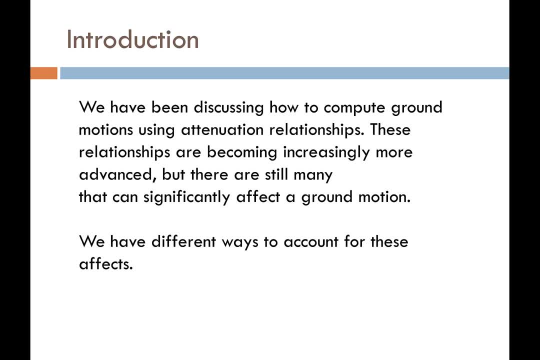 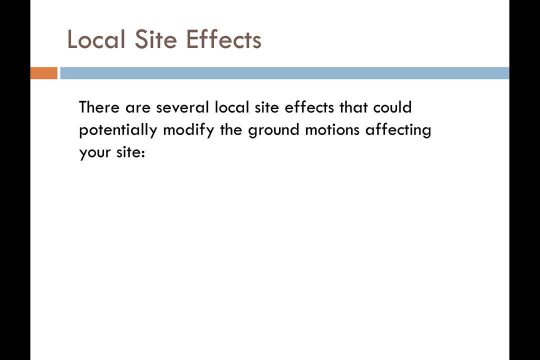 Attenuation relationships are getting better at accounting for more of these side effects, But to date we still have to perform separate analyses to account for a lot of these effects. So let's just jump into it. We're going to discuss local side effects today that can significantly affect ground motions. 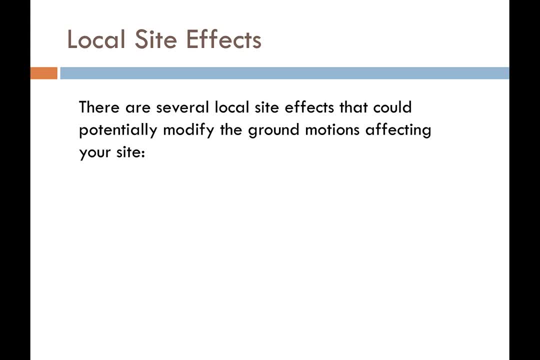 So what are the side effects that we're going to discuss? And, by the way, before I jump in, I am recording this from my house, in my kitchen, and I've got lots of kids. I've got six kids and they're going to be coming home from school here soon. 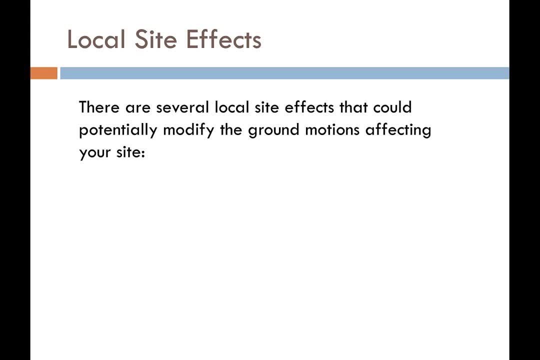 So it might get a little bit crazy. My dog might bark. If that's the case, just smile and laugh and move on, because this is all part of the craziness that I and you and everyone else is dealing with in this COVID pandemic. 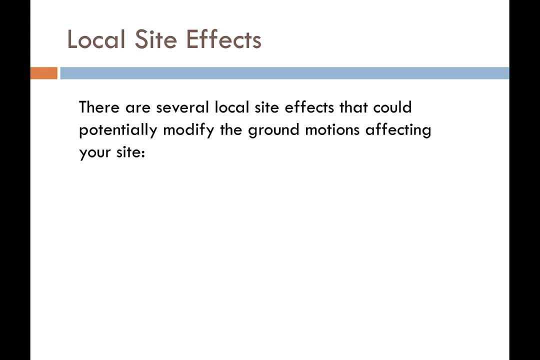 Here are the local side effects that we're going to talk about: Soil amplification or site response, near source effects and directivity, topography, or topographic effects, and basin effects. So each of these, we're not going to dive very deep into each of these to the sense that you're going to be an expert. 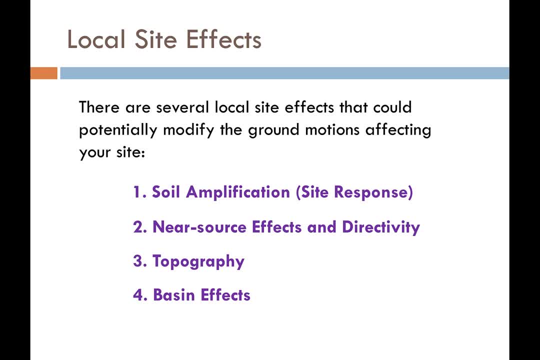 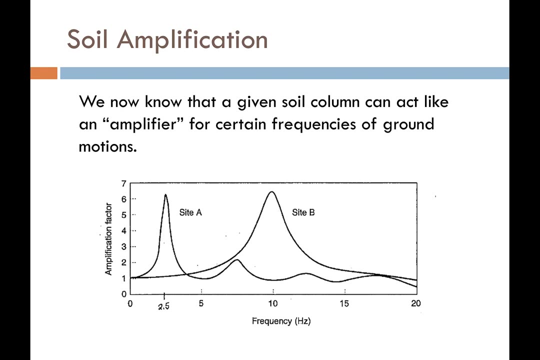 But I'm just going to teach you enough to make you dangerous, And just so you understand the concept, because even just understanding the concept is incredible. It's incredibly important in decision making today. So let's discuss soil amplification. But I think the easiest way to understand our soil amplification is if we just look at a whiteboard. 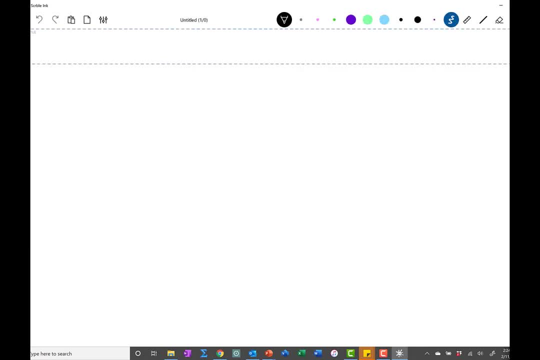 So I'm going to delete what I had on there before And let's just- let's just do a simple comparison. OK, let's just say we have the actual And then we have the model. So for the actual, I have some bedrock. 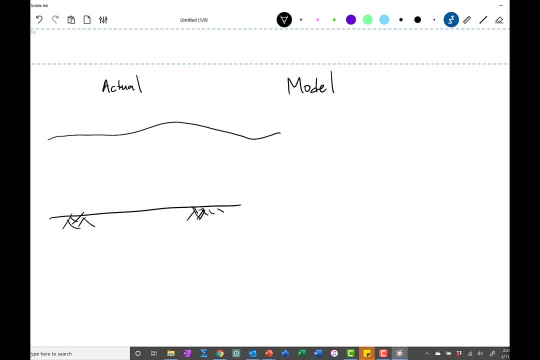 And on top of the bedrock I have maybe some soil. It might be level and might not. In fact, let's just for simplicity's sake, let's assume it's level And then I subject this bedrock To some sort of ground motion. 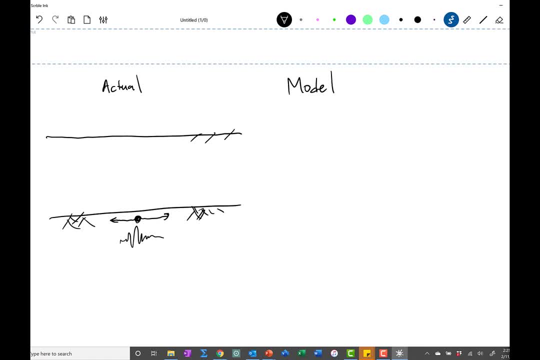 So there is an earthquake, that happens, The bedrock shakes horizontally and vertically, back and forth, up and down, And those motions transmit all the way in. at the ground surface There is also motion, But that motion that occurs at the ground surface might be different than the motion and the rock. 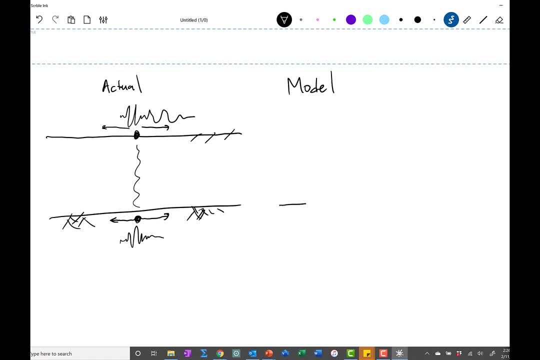 And why is that? Well, because we can see why if we just draw a model. So let's say I have rock or a table, And on this table I have a spring. I've never drawn a spring before. I think that's pretty good. 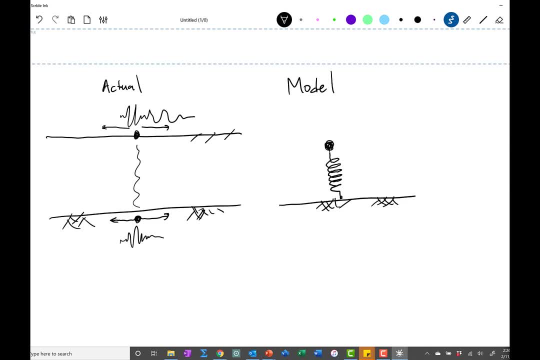 And on this spring I have some Mass And, let's say, the same thing happens. So I shake my table according to some ground motion And then my mass also will respond in some way. It will have some different motion And that motion is really a function of the spring that that mass is sitting on. 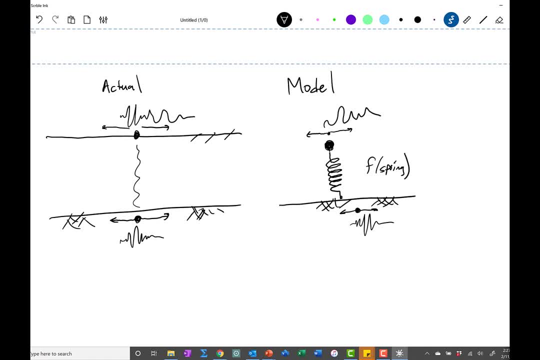 It's also a function of the mass. It's also a function of the mass, of course, But this spring is going to have a natural period or a natural frequency that it vibrates at, And so understanding how motions are transmitted from the table or the rock through the spring up to the mass at the top of the spring. 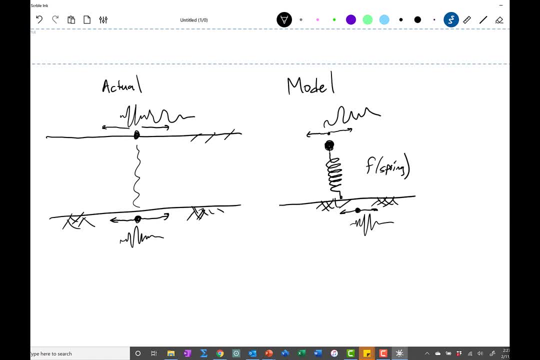 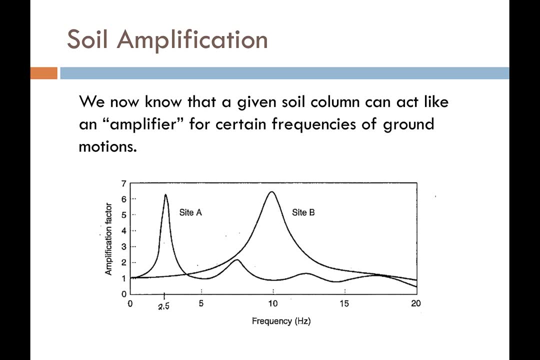 that is what we're talking about when we say site response. All right, So going back, Soil amplification or site response, If we look at how that spring or how that soil can amplify the base motions in the bedrock, this figure right here shows the amplification that happens at certain frequencies. 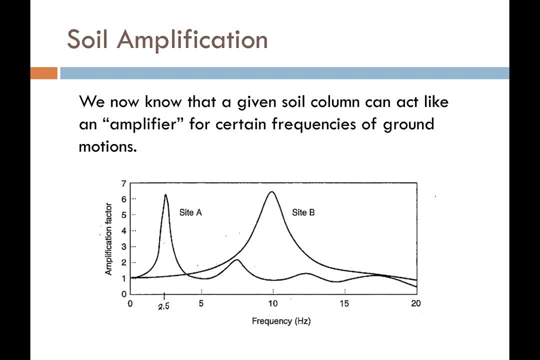 depending on the stiffness or the natural frequency or natural period of that spring or the soil. So here at, for instance, site A, we could say, OK, maybe this is a really This is a softer site because, notice, at a low frequency it or it is amplified quite a bit. 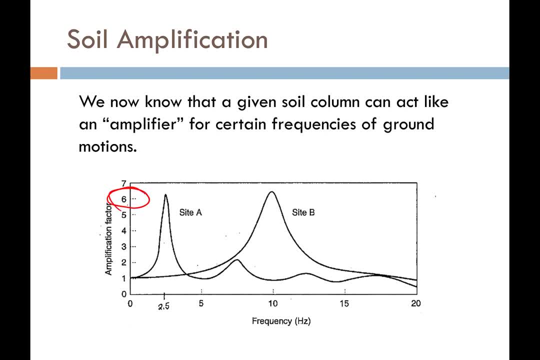 And how much is it amplified? Well, it's amplified greater than a factor of six. So that means that ground motions in the table that are at the frequency Of two point five hertz that go into that spring or that soil when they come out the other end. 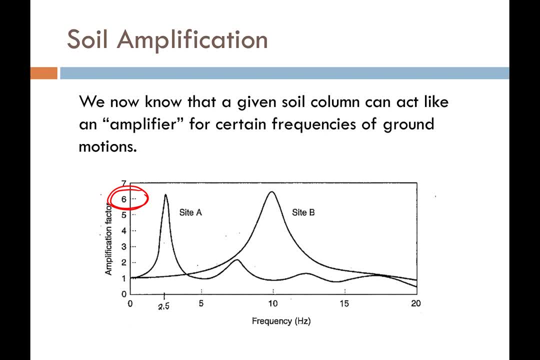 those are amplified by more than six hundred percent. That's pretty crazy when you think about it. Can we have the amplification? Yeah, sure. So check out what's happening down here at, say, a frequency of 20.. So that's really high frequency stuff. 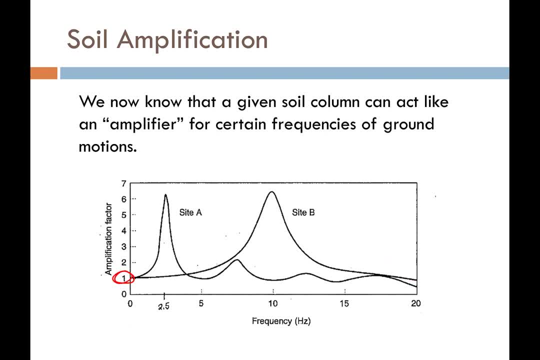 It's less than an amplification ratio of one. So anything that's less than one, Anything that's less than one, is getting filtered or de amplified. for my second site, here Say, I have a totally different site, a totally different representative spring that may amplify at a different frequency. 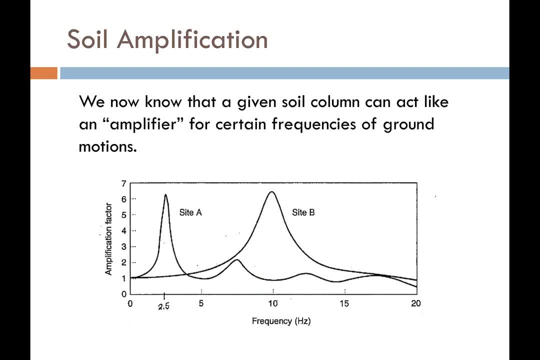 In this case, 10 hertz. So all that's saying is that site B tends to resonate at a frequency of 10 hertz and site A tends to resonate at a frequency of two and a half hertz. So understanding how different sites resonate, understanding what their natural periods or natural frequencies are, will help us predict soil amplification. 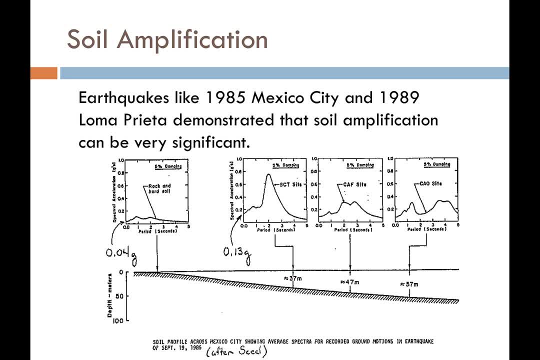 This is a really important lesson to learn And there was no event that taught this more effectively to the earthquake engineering community than the 1985 Mexico City earthquake, And I was heavily involved, And I was heavily involved in the earthquake reconnaissance following the 2017 Mexico City earthquake. 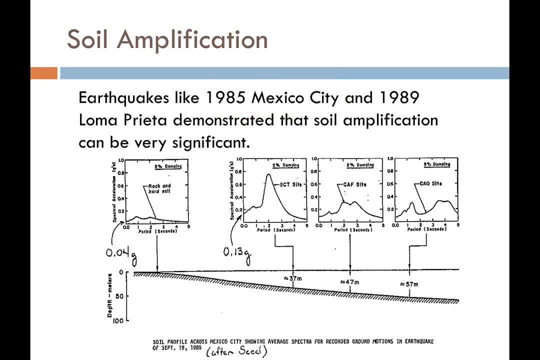 And we saw the exact same stuff happening. Here's what happened in Mexico City in 1985.. An earthquake occurred well over 100 miles, almost 200 miles, away from Mexico City, And those ground motions traveled all the way to Mexico City. 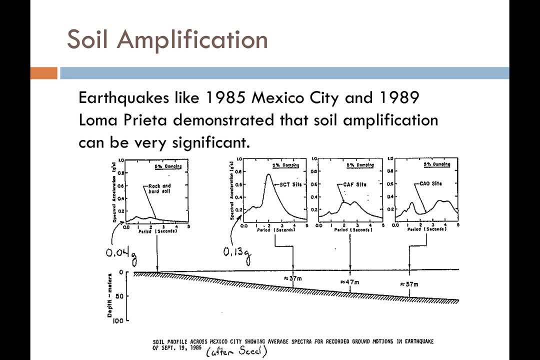 And they entered the Mexico City Bay Area. They entered the Mexico City Basin through the rock that lays beneath it, And the motions themselves were pretty darn small, In fact. here's the response spectrum that was recorded of the ground motions in the rock. 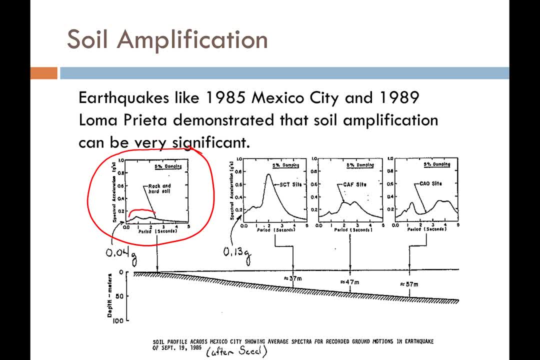 And you can see that the peak motions occurred between a period of one and two seconds. generally Looks like there were almost two peaks, So it was bimodal. So it was bimodal And the peak accelerations were just a little bit over 0.1 g. 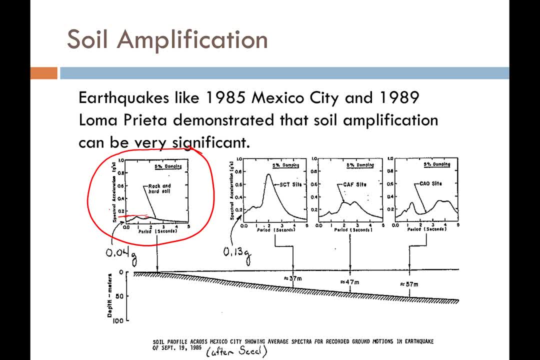 So you know, 10% g, That's pretty small. In general. that would not damage many structures at all in modern construction today, Especially in a modern city like Mexico City. But the freaky thing is Mexico City has this stuff in here. 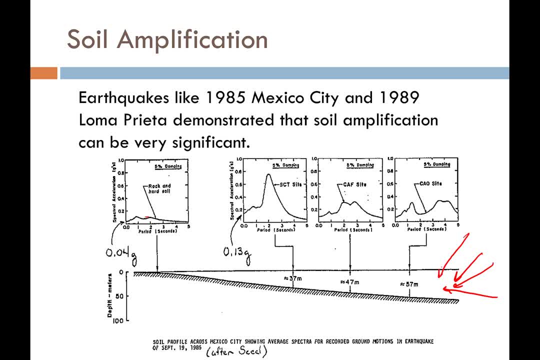 Freaky, soft, gooey clay That comes from an old lake that was called Lake Texcoco. The lake is largely not there anymore. I think there's a teeny little remnant of it left, But that clay is mucky. 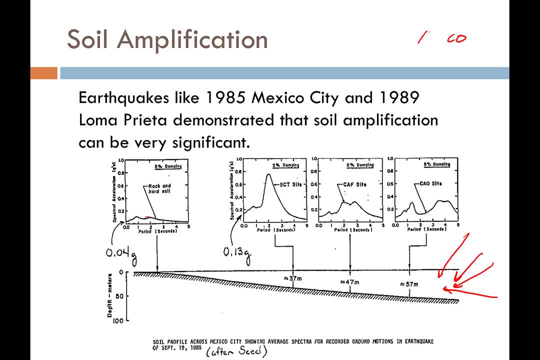 It is soft, It is sticky, It's gooey And to a geotechnical engineer it's like Christmas, Because it's just fascinating stuff. Anyway, this basin in Mexico City is filled with this gooey clay And there were several ground motion recording instruments located throughout the Mexico City basin. 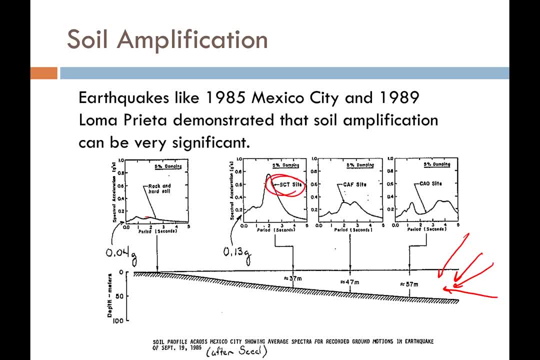 There was one located in this location. If we just do a cross-section across the Mexico City basin. There's one in this location, There's one in this location, And then there's one in this location, And each of these have different names. 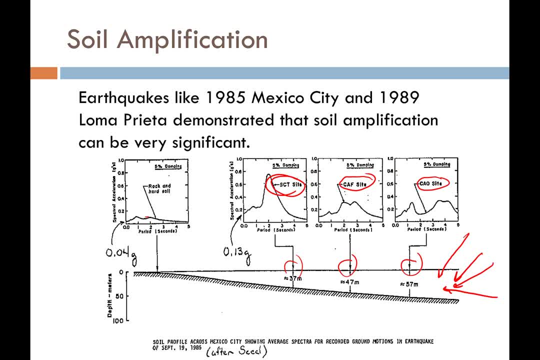 SCT, CAF and CAO: These are the names of the ground motion recording stations. Oh, hold on, Hey, Chad, I'm recording a lesson. Can we be quiet? Awesome, Thanks, All right, So check out the response spectra from each of these stations. 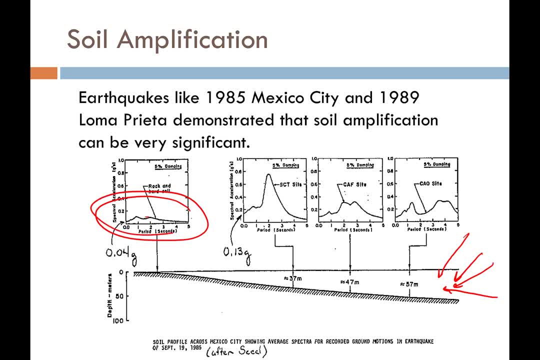 So, even though the same input went in beneath the soil in each of these locations, the output was drastically different. Here, at this location of about 37 meters of thickness of that gooey clay, here's the response spectrum that resulted, And what we see is that, at a period of around two seconds, there was massive amplification, to the point where we almost had about 0.8 g of acceleration at that period. 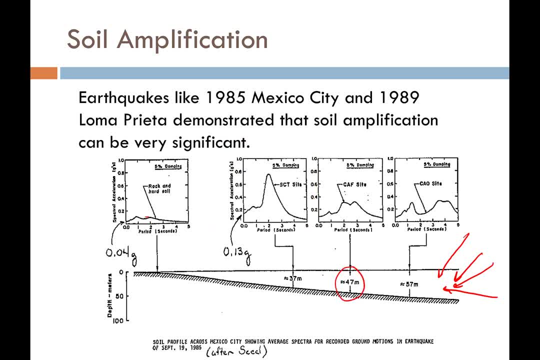 And as the clay got thicker, the spring- this model spring- got softer and softer and softer. So it started to amplify at increased speeds. So it started to amplify at increased speeds. So it started to amplify at increasingly higher periods. So it started to amplify at increasingly higher periods. 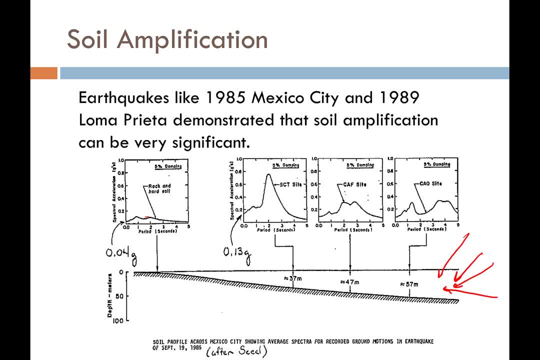 So it started to amplify at increasingly higher periods. And so you can see, now the peak is about two and a half to three seconds. And so you can see, now the peak is about two and a half to three seconds. And so you can see, now the peak is about two and a half to three seconds. And then here, where the clay is even thicker, about 57 meters, that spring is really soft. And then here, where the clay is even thicker, about 57 meters, that spring is really soft. So now we start to see kind of two peaks start to develop. 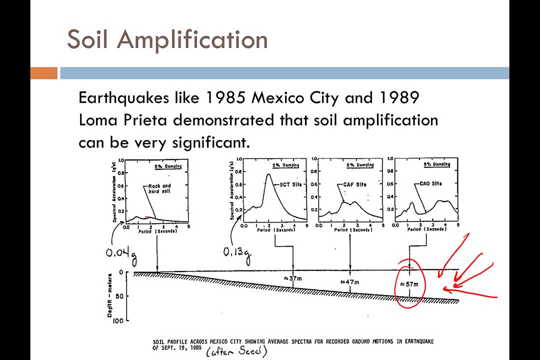 So now we start to see kind of two peaks start to develop And the amplitude of these peaks is much less than the peak over here And the amplitude of these peaks is much less than the peak over here And the amplitude of these peaks is much less than the peak over here. 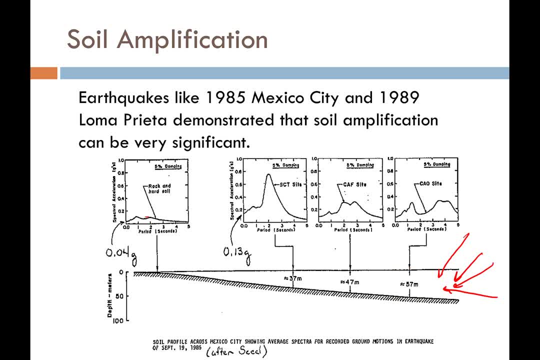 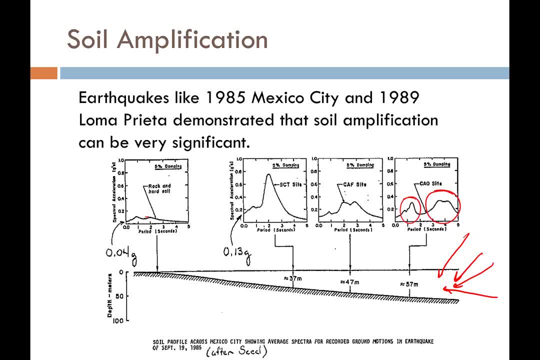 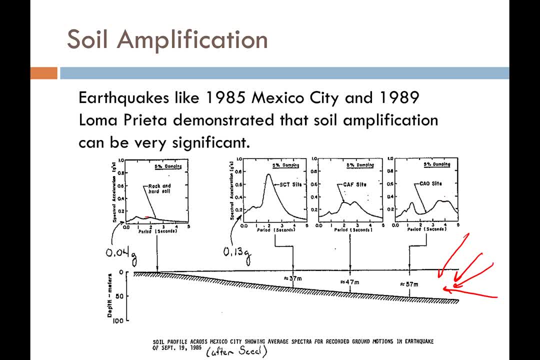 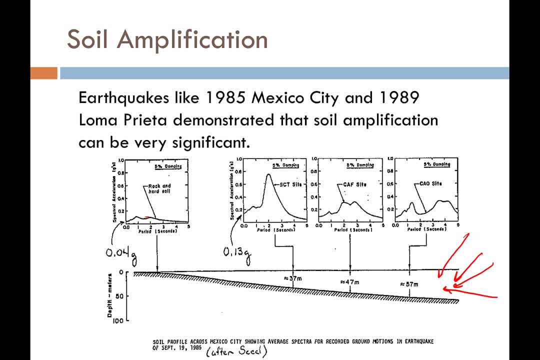 less than the peak over here, but still. i mean here we are at about a period of four seconds. so what does that mean? well, in a ring, or in certain sections of mexico city, and it kind of formed the shape of a ring, which makes sense because it happens where the soil is right around. 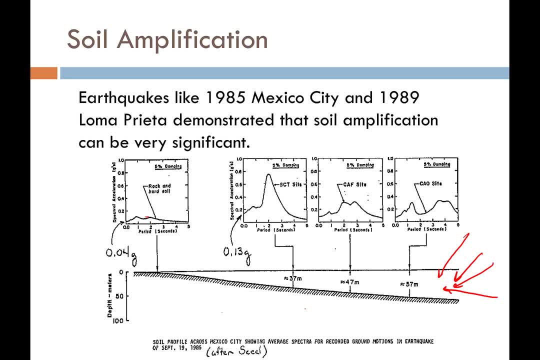 40 meters thick. we got this big spike at about a 0.2 second period and, interestingly, buildings that are between about 12 to 20 stories in height, somewhere around 15 stories in height. guess what their natural period is approximately? yeah, it's about the same as that peak, so um now, 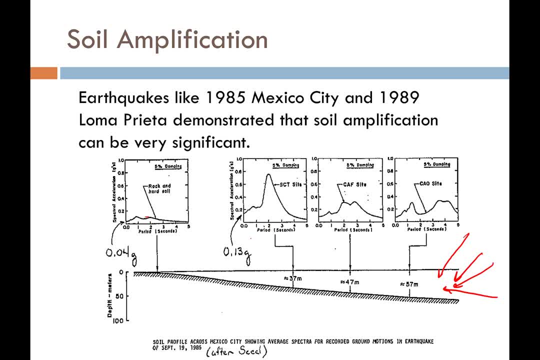 you're. you're in trouble because your building is in tune with the soil and the soil is in tune with the earthquake. everything's in tune. and now you start to really shake and rattle and destroy these buildings, so buildings that were in this region where the soil was about that thick and 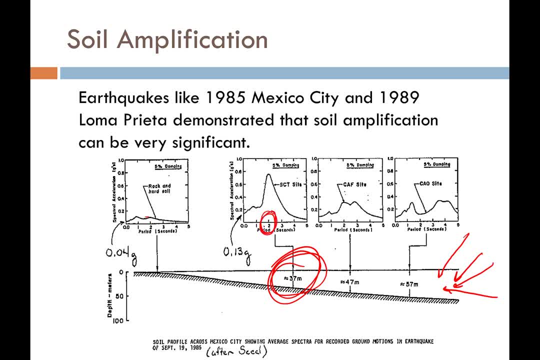 that had natural periods around point, around two seconds. uh, they collapsed and it killed a lot of people, thousands of people. but we learned an important lesson from this tragedy. we learned about soil amplification and site response, and this earthquake, followed by the loma prieta earthquake in california four years later, really kicked off a ton of research in the area of site. 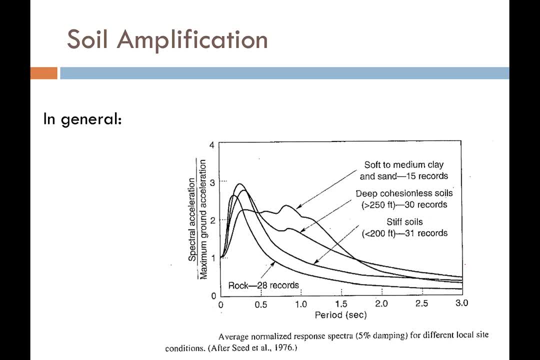 response. so here's the things that, uh, in general, we can state, okay, that these curves here or curves here on the earth are not necessarily the same as the one i mentioned before. we can, you know, get rid of them and use a little more, a little more of the terrain. you can get rid of them and get rid of. 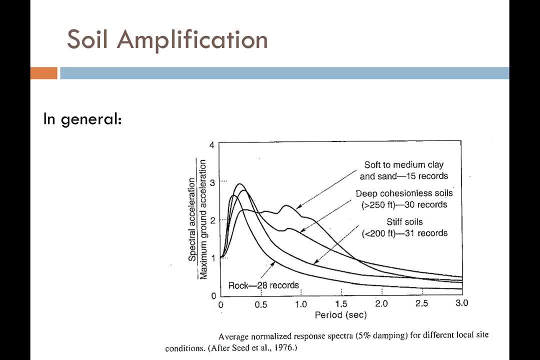 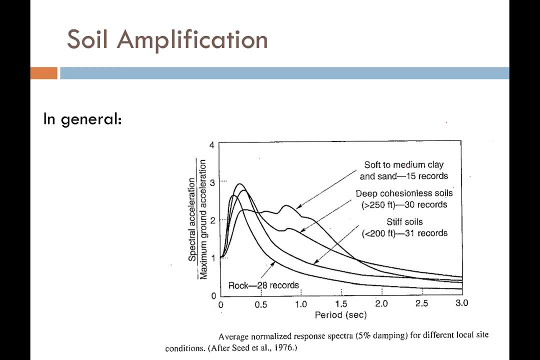 just kinda one-off. it's simply the bike of the earthquake. i think we'll be able to get to that point. so now let me talk a little bit about the year 2019 and what it was. developed by thick cohesion lists, or sandy soils, and 31 records on very stiff or dense soils. 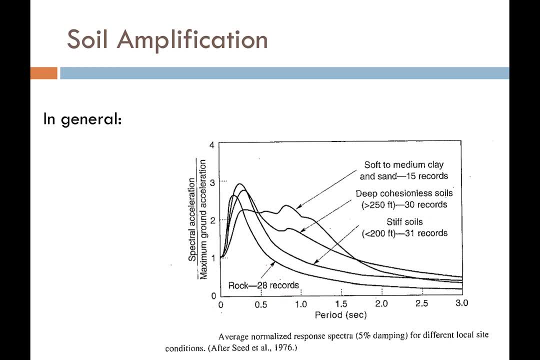 and then he had 28 records on rock and what he did was he just computed the, the mean or the average response spectra from all of these records in their respective categories and we see that the rock rock has a its peak at a much lower response or a much lower period. excuse me, so that means that it tends to 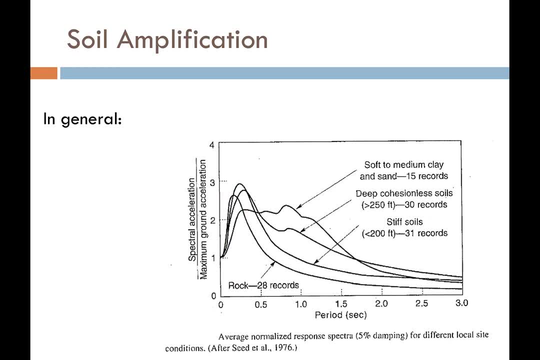 resonate at higher frequencies and it's really stiff soil. it it's a resonates at a little bit higher period than rock, but it still has a similar shape to rock, except notice that there is quite a bit of amplification relative to the rock, and then the softer, we go all the way out to the soft and medium clays we tend to see. 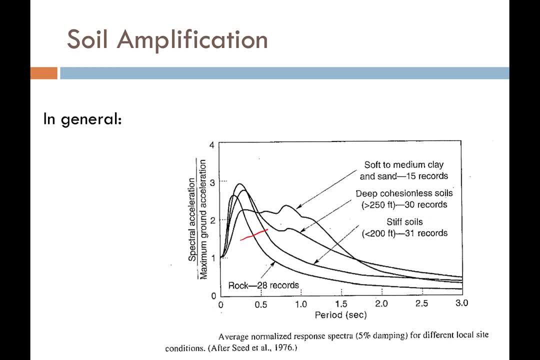 that the response spectra stretch out in this direction, such that high period stuff, stuff that greater periods greater than half a second to greater than one second. those are the, the periods that really start to get amplified. and so the the lesson that harry seed really tried to teach the world is that site response matters, the. 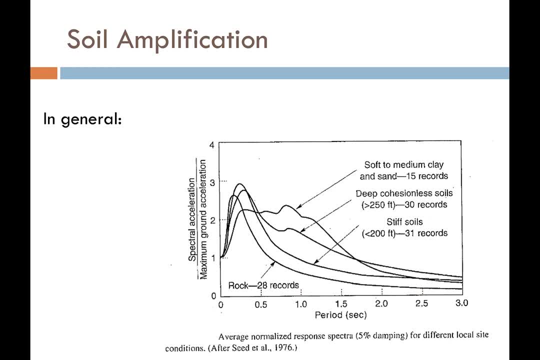 types of soils that you build on matter. not all soil is the same and it doesn't just depend on the fault and the size of the earthquake, but it depends on the soil that you're built on as well. so, in general, softer soils are going to amplify high period ground motions and harder 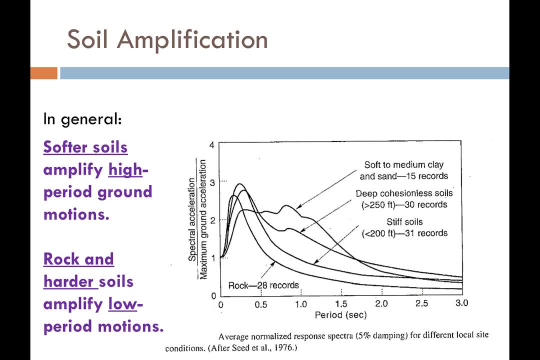 soils or stiffer soils and rock are going to amplify low period ground motions and the the the opposite is true. rock and harder soils are going to filter or de amplify high period motions and soft soils are going to filter or de amplify low period ground motions. so how do we? 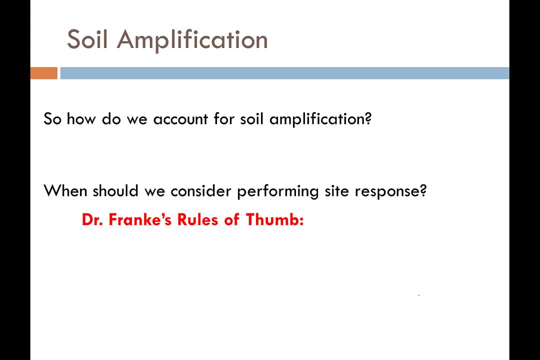 account for soil amplification, couple of things. well, the the analysis that we do is called a site response analysis, and we're going to dabble with site response analysis a little bit later in the semester, but for the time being, we're just going to learn about it. so, as an engineer, when should you consider? 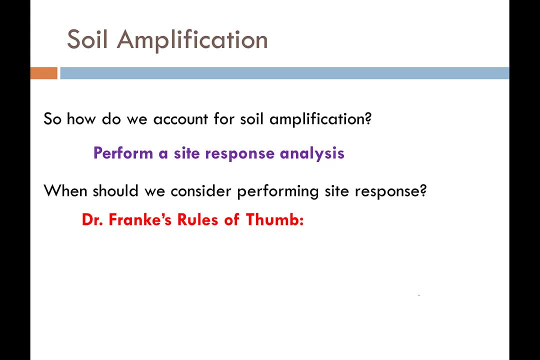 performing this type of analysis. well, here are my rules of thumb that I would use in my own practice. the first is whenever I have a structure whose natural period is greater than half a second and the average shear wave velocity in the soil in the upper 30. 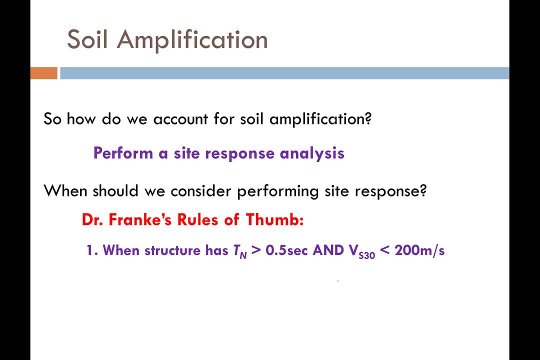 meters or the upper hundred feet is less than 200 meters per second or so. the second is if I have a structure whose natural period is greater than half a second And I have any soil layer in my soil profile that has the potential to liquefy across my site. 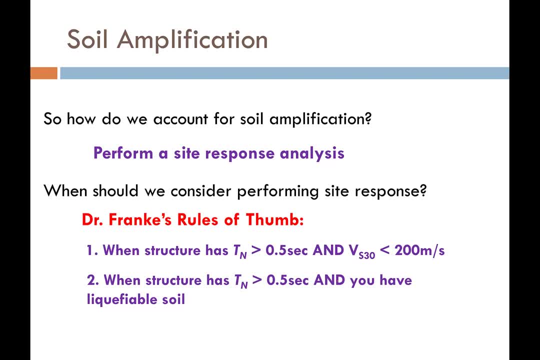 And the reason that is the case is because, even if I have a thin soil layer- that's maybe two feet, three feet thick- and it liquefies, it acts like a giant filter And it will amplify the ground motions even though it's only a couple feet thick. 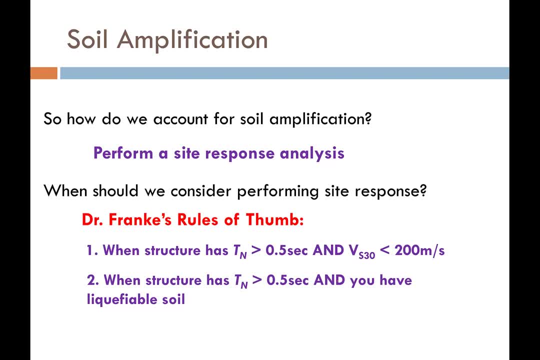 It will amplify those high-period ground motions and filter out the low-period ground motions or the high-frequency stuff. Third is any time you have any critical structure built on soil and your average shear wave velocity in the upper 30 meters is less than about 270 meters per second. 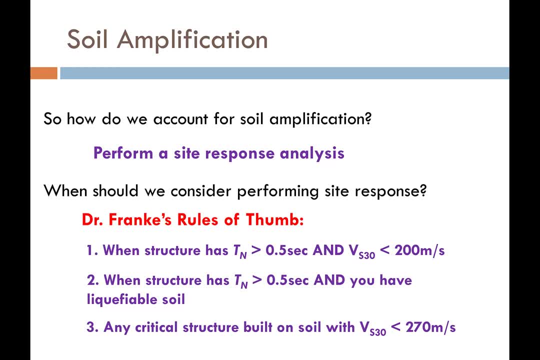 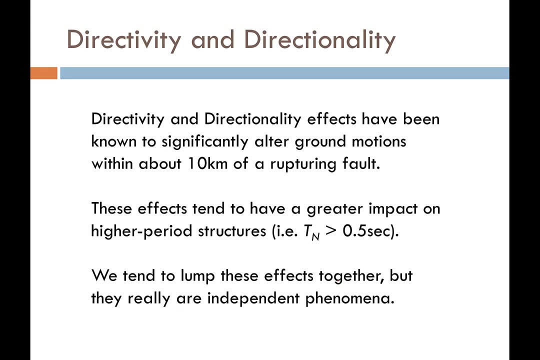 Now again, this isn't written in code anywhere. This is my own personal experience. Just learn through practice, and those are my rules of thumb. Okay, let's go to the second one. This is directivity and directionality. Now we've talked a little bit about directivity earlier in the semester, when we compared it to the Doppler effect. 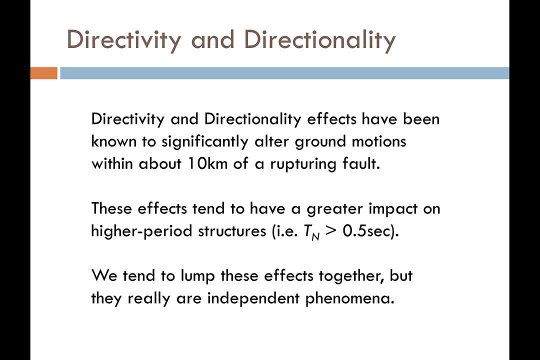 And so you can go back and learn more about it in that lecture, But Because we're going to talk a little bit more about what it looks like to account for it in your ground motions. So directivity and directionality, it's important. 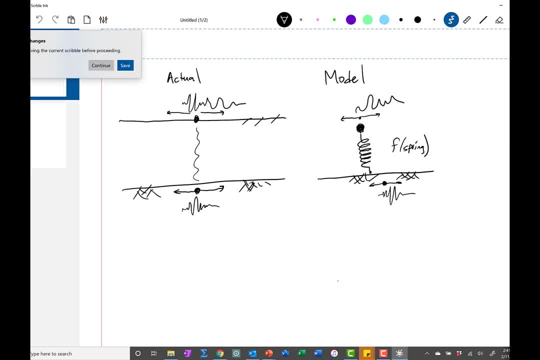 Maybe what I'll do is just model for you what these are again. So if I have a Say, I'm a bird and I'm looking down on the ground and I have a fault that runs like this. So this is in plan view. 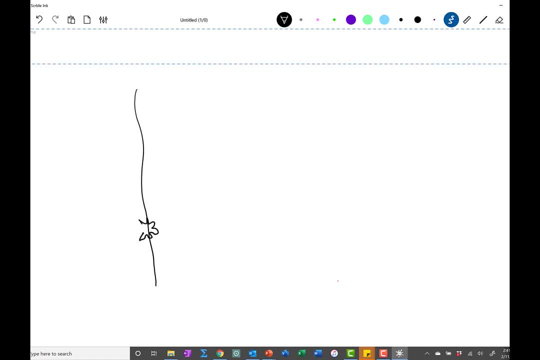 And let's say that The fault ruptures right there. It looks more like a flower than a rupture, but there you go, All right. So if the fault begins to rupture right there and the rupture propagates along the fault, What's going to happen is, every time that rupture propagates as the fault breaks and as disparities break. you get the breaks along the fault that just start happening as that rupture propagates along the fault. And every time the rock breaks it releases more and more and more waves. So this is going to look messy here pretty soon. And so all those waves. 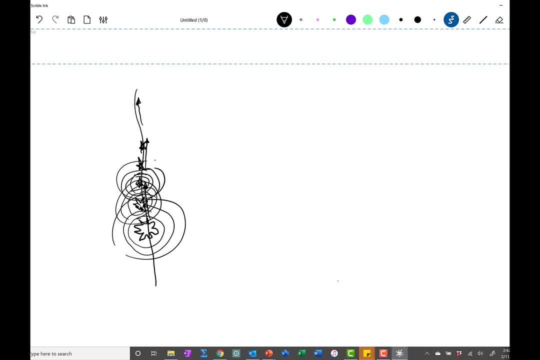 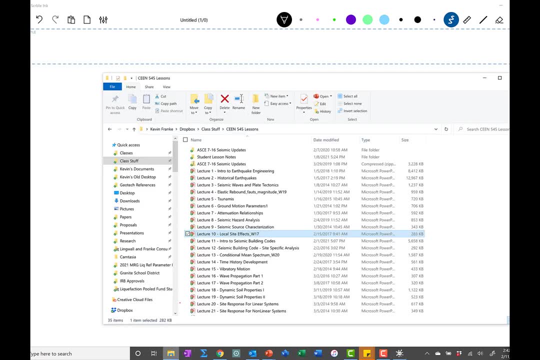 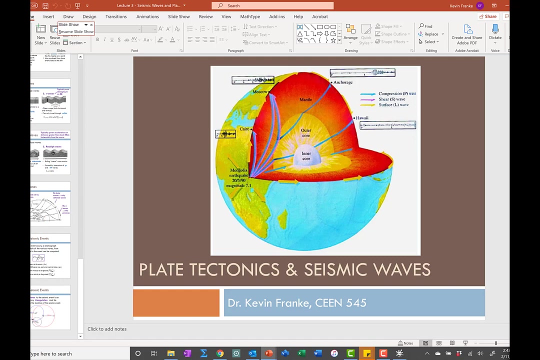 Just continue to propagate and move, And what ends up happening, if you'll recall, is what we showed. I think it just made more sense if I just show it to you. Is it in this lecture here? No, Next one, Next one. 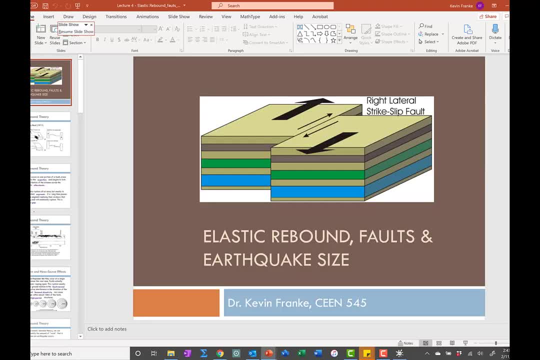 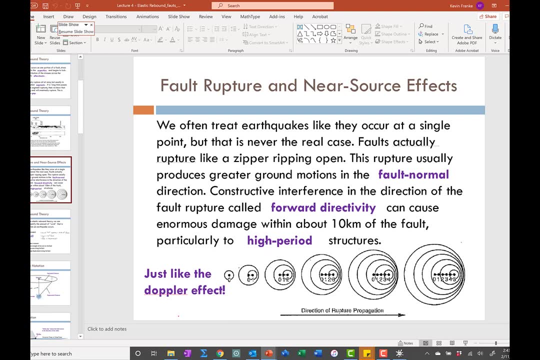 I could try to draw the figure. I could draw the figure for you, but it's not going to look very pretty. Yeah, here it is, This one, right here. So this figure right here demonstrates really well what's going on with directivity. 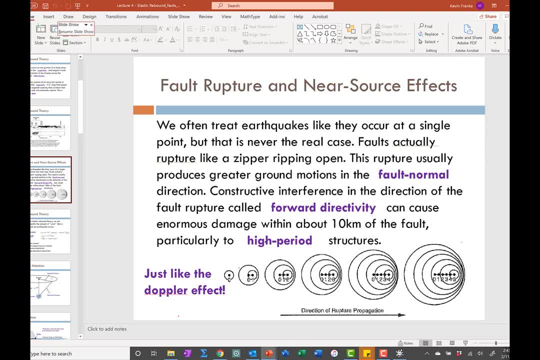 So every time new rupture occurs and new waves are emanated in the direction of the rupture, you get a big stacking of energy. And that stacking of the energy, just like the Doppler effect, changes the, in essence the frequency of that loading. 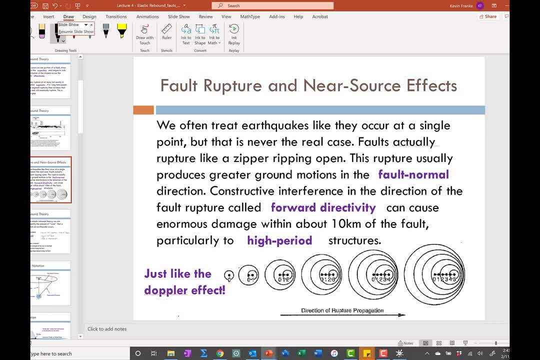 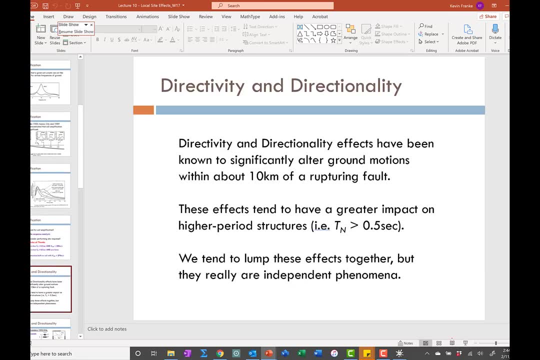 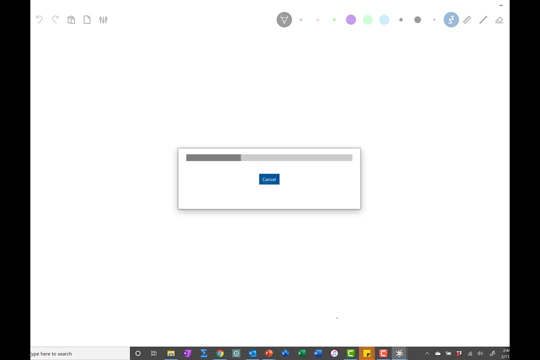 And it can also affect the intensity or the amplitude of it, And so that big pulse of energy can cause a tremendous amount of damage. So that is the, That is the, That's directivity. Now, If I go back to my messy drawing and I just erase everything, 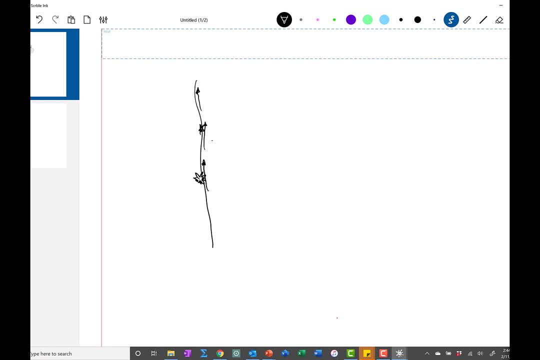 and we get back to one little earthquake. Now, if I look at just one break and the waves that are emanated from that break, If I had, let's say, recording instruments that were that were, that were oriented in different orientations, 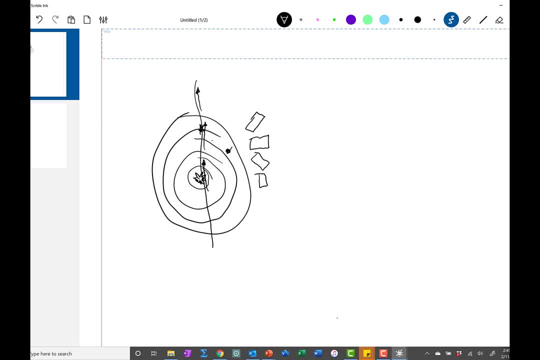 Let's say that I had a location right here and I had all of these instruments located right at this one location, okay, And they were all oriented in different, in different orientations, And I were to draw the response spectra for all of these different instruments. 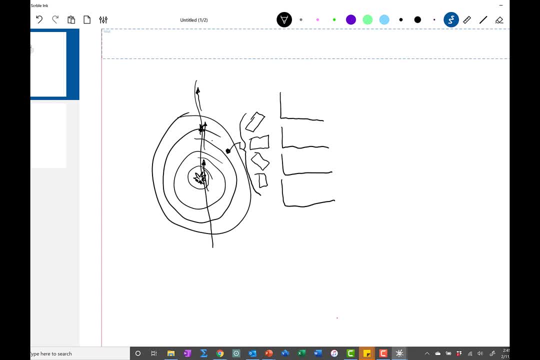 Here's the crazy thing. So these are period T on this axis and then on this axis. this is spectral acceleration G. What I might see in each of these would be: You would expect them to be very similar because they're in the exact same location, recording the exact same earthquake. 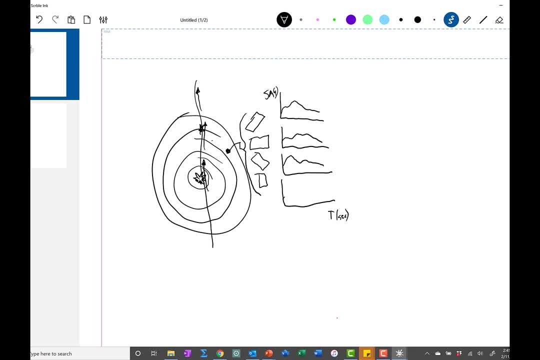 But they're not going to be similar. In fact, depending on the orientation of the instrument, I'm going to record a different ground motion, I'm going to record a different earthquake, And so the orientation that I'm recording those ground motions. 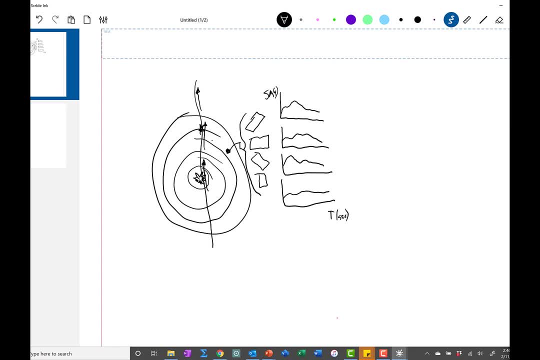 or maybe I should say the orientation of the earthquake waves themselves. that's what we call directionality, And in one of these orientations there's going, And at each period there's going to be an orientation that gives me the maximum peak at each period. okay, 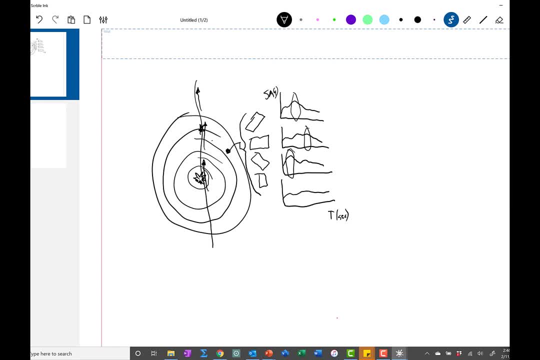 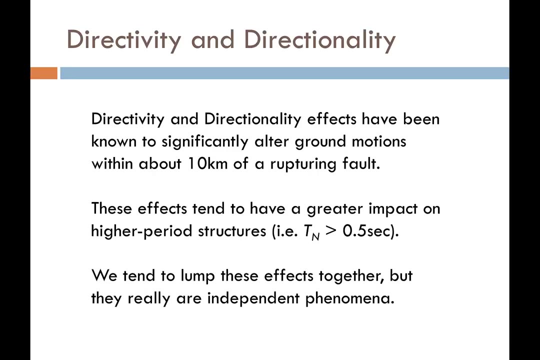 And so each period in my response spectrum has an orientation that has a different maximum amplitude in the response spectrum, And so, as an engineer, I may be interested to know which orientation is the maximum orientation. So we tend to consider these effects, directivity and directionality, together. 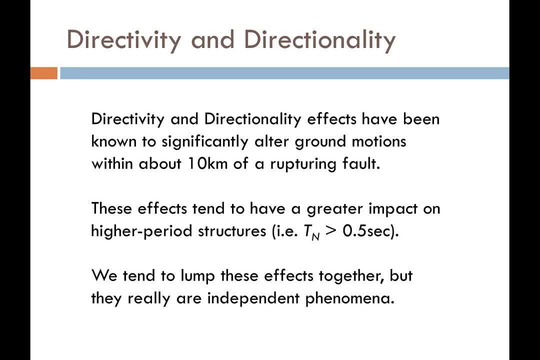 We lump them together and call them. I thought I had that written, but I don't, so I'll just write it in here. We tend to call these things near-source effects, So if you ever hear this phrase, near-source effects. 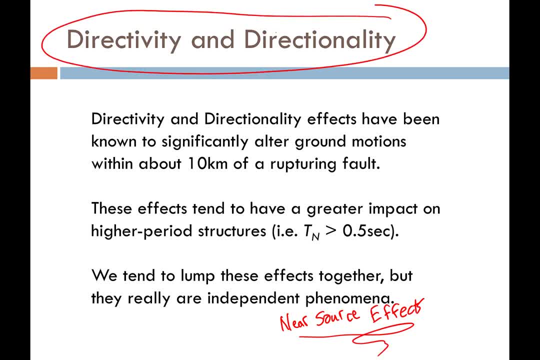 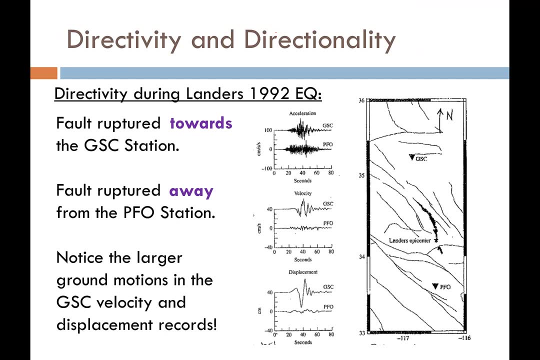 we're referring to directivity and directionality usually lumped together, but they really are two different phenomena. So let's look at some real-life examples. When I deal with directivity, I can have forward directivity so it's in the direction of the fault rupture. 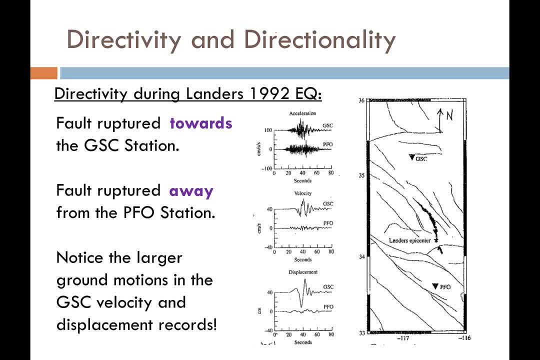 or I can have backwards directivity which is in the direction opposite or away from the fault rupture. So here's one example of recorded ground motions. This is the Landers 1992 earthquake in Southern California. The earthquake started right here And it largely went in this direction. 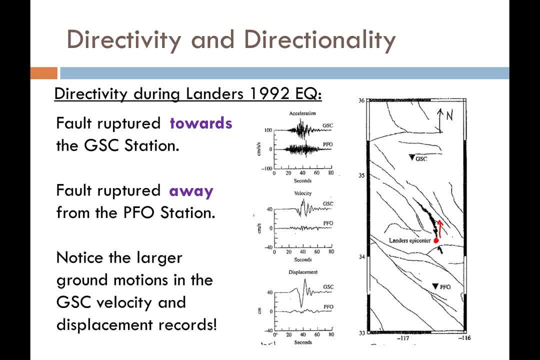 It went to the north. Now I've got a station located to the north called GSC, and then I've got a station located to the south called PFO, And each of these they're about almost the same distance away from the rupturing fault. 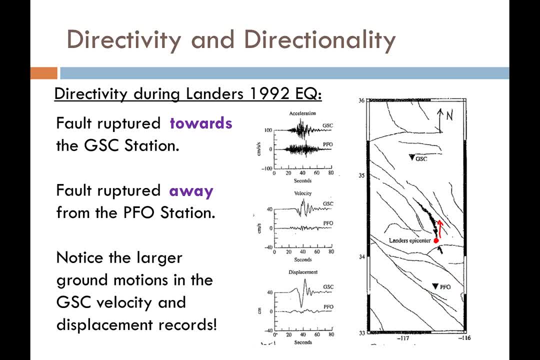 And so they recorded ground motions, But the ground motions they recorded, even though they're about the same distance away, are drastically different. Here's the accelerations that were recorded at GSC, And here are the accelerations that were recorded at PFO. 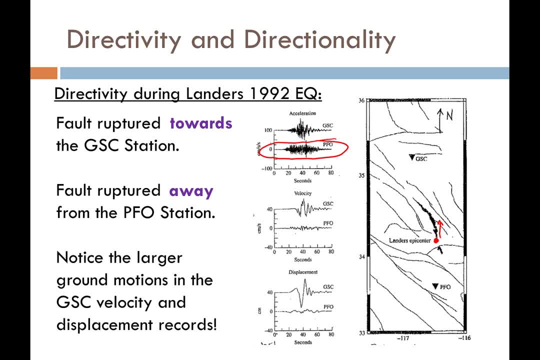 And they look like totally different earthquakes, don't they, when you look at them? Look at the velocity records. The velocity records we see GSC has a big peak And And PFO, nothing, Just kind of wiggles. 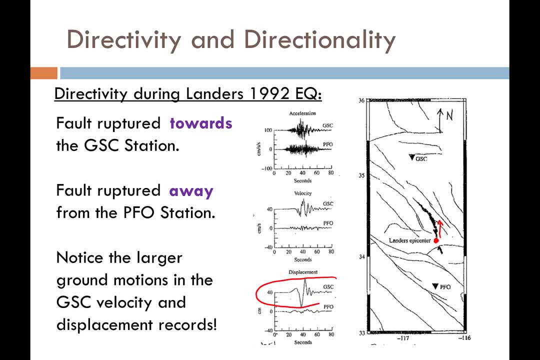 And in the displacement records. yeah, there it is. GSC has a velocity pulse, Okay, And a PFO or a displacement pulse, excuse me, And PFO has nothing. So these pulses, you guys are what we call directivity pulses. 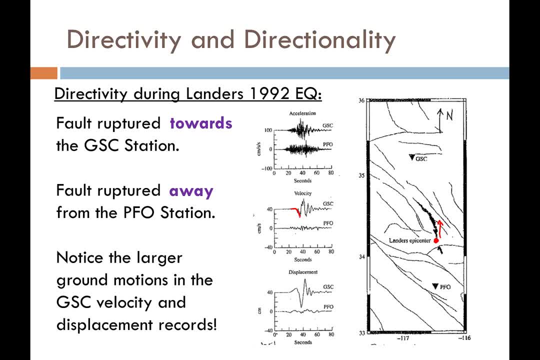 And they have a little, usually blip down, a big jump up, And we tend to see them blip up, big drop down. We tend to see them in the velocity and the displacement time histories And it's these pulses of velocity and displacement. 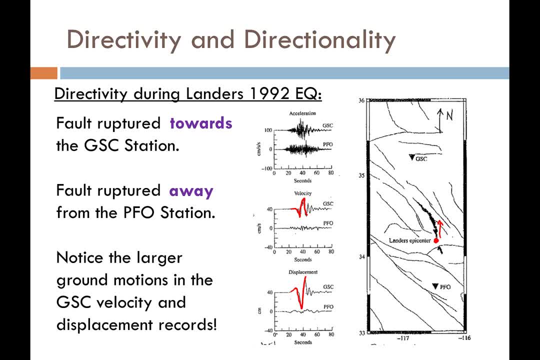 that just wreak havoc on a lot of infrastructure, especially anything that has a higher natural period of frequency or a natural period of vibration. So, in general, forward directivity is the scary thing that we worry about with directivity, But one thing that we can't ignore. 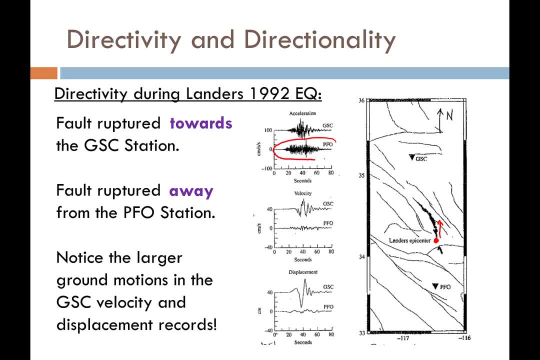 is that the duration tends to be longer in backward directivity. So, even though the amplitude of our intensity, the amplitude of our motions, is not as great as it is with forward directivity, the duration of the significant loading is stretched out. It's stretched out longer in backward directivity. 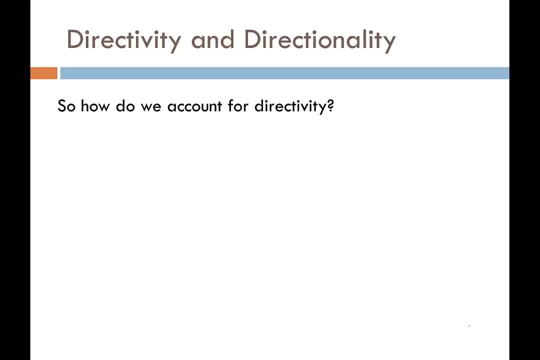 Okay, so how do we account for directivity? That's a really good question There's. it's obviously something that's important And, depending on what our structure is- whether it's a long period or a short period structure- we will want to look at both forward directivity and backward directivity. 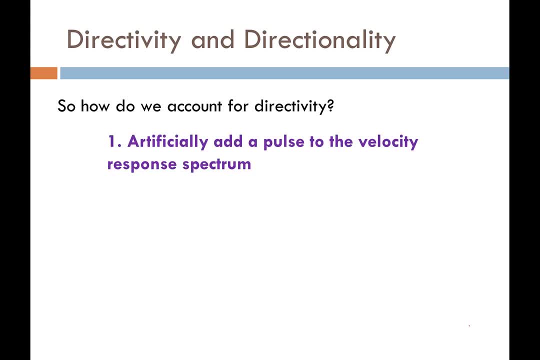 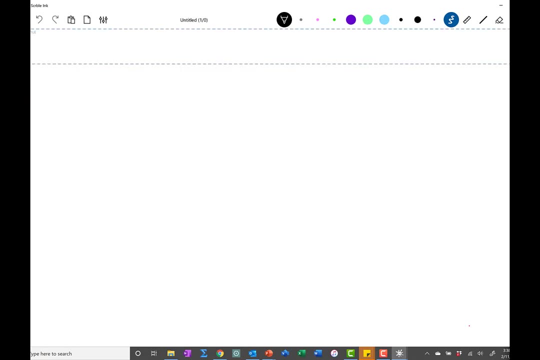 So how do we account for it? Well, one thing we could possibly do is add artificially a pulse to the velocity response spectrum. So I'm not sure if you guys have done this yet, but in seismosignal you can plot, of course. 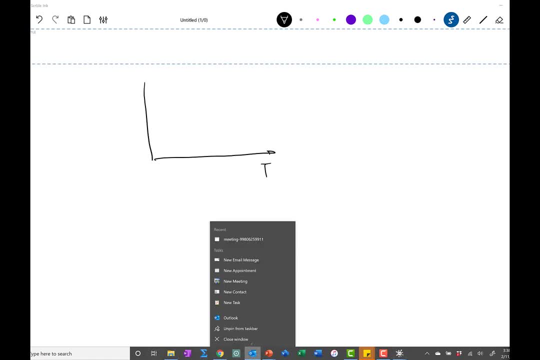 let's turn off my emails. There you go. You can plot spectral acceleration and those will look. you know something like this. But you can also plot spectral velocity, And spectral velocity will always look something like this, And and so what we could try to do. 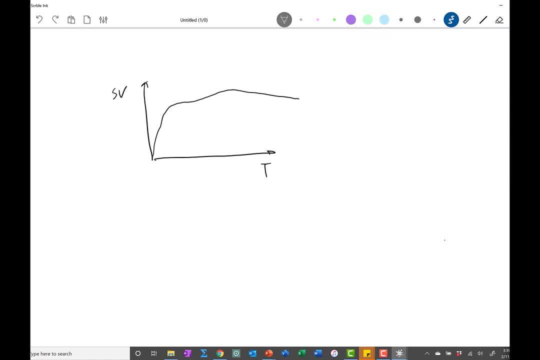 is, we could try to come into the spectral velocity plot and artificially adjust it so that for the appropriate periods that are high we could try to modify it to properly account for that pult that we saw in the velocity time history. And yeah, that sounds great. 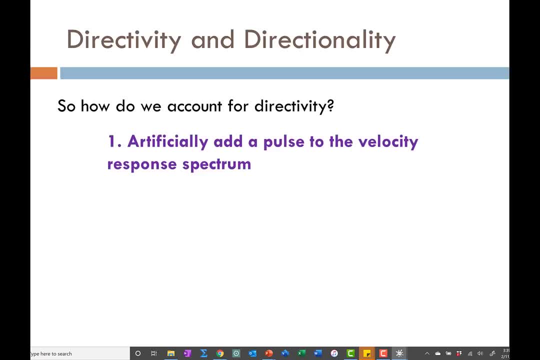 The problem is that to modify that velocity response spectrum is pretty tricky to do And it's even trickier to do correctly. There we go, And so, and the reason for that is because we don't want to just throw numbers in there willy-nilly- 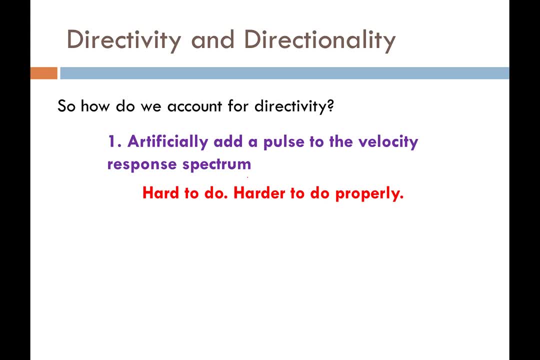 We want to put numbers in there that are realistic and numbers that are representative of actual earthquakes, So we can go to our, we can do it empirically and we can look at earthquake records and things, and that's fine, That's something that we can do. 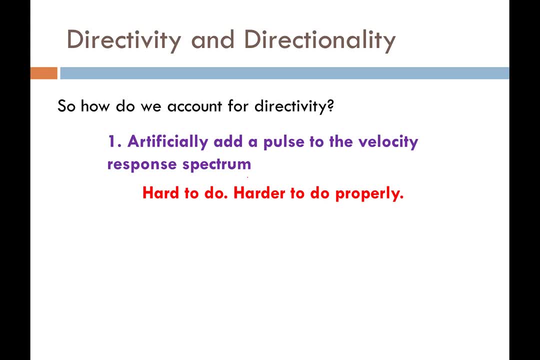 But it's just not done by a lot of people. So another thing that we could possibly do is if we were using, we were doing some sort of dynamic analysis like a site response or a structural dynamic model, and we were requiring earthquake time histories. 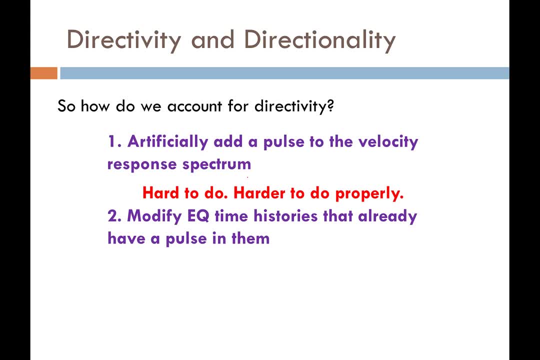 then we could just select time histories that already have these directivity pulses in the recording. So these ground motion instruments experience that directivity pulse, And so we can just use those and run those through our model, whatever the model is, And so this is a really popular approach. 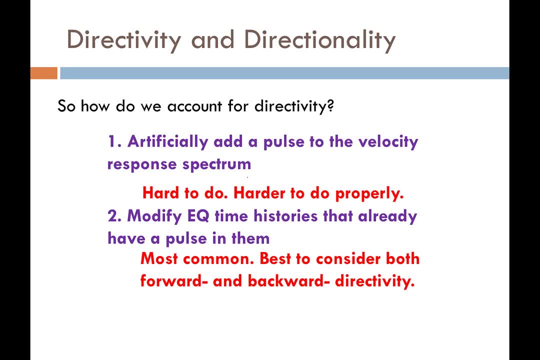 It's very common, And when we do that and we're selecting time histories that have directivity in them, we want to make sure that we're selecting time histories with both forward directivity and other time histories that have backward directivity, Because, again, 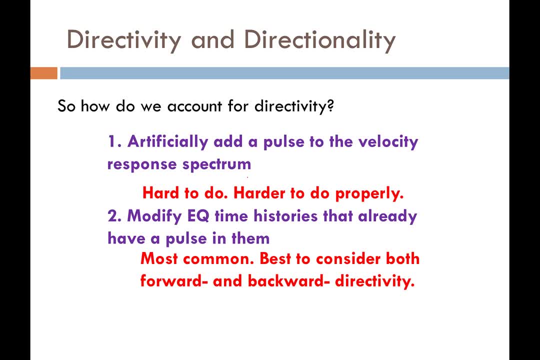 the forward directivity gives you the big kick in the higher periods in terms of velocity and displacement, But backward directivity usually has longer duration, And so we want to account for them. And then another thing we can do is simply apply these directivity multiplier functions. 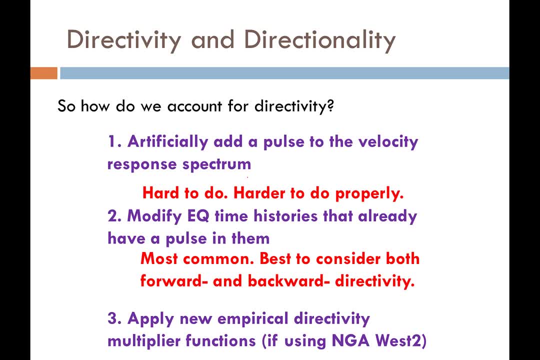 to the acceleration response spectrum, And this is also very popular. It's very common to do This. may sound a little bit like the first one, but for whatever reason, we're more comfortable modifying the acceleration response spectrum than we are the velocity response spectrum. 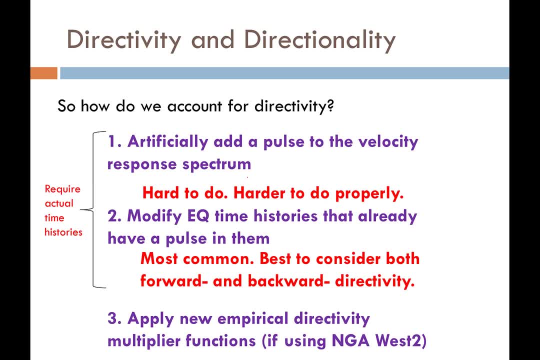 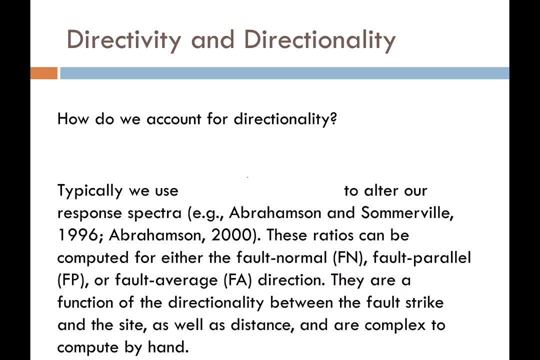 So note, by the way, that the first two they do require actual time histories. The third doesn't, And that's one of the reasons that it's pretty popular. So I've usually done the third one myself a lot in practice. 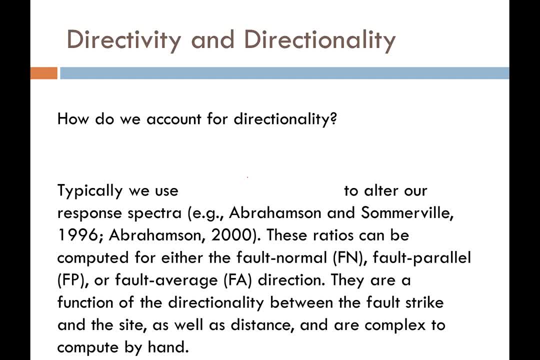 Let's talk a little bit about directionality. So when we talk about directionality again, this is how the intensity of the ground motions change, depending on the orientation of the ground motions relative to the rupturing fault. Now, typically what we're going to do, 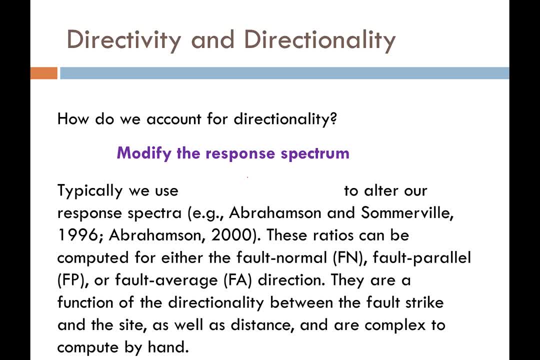 is we're going to modify the acceleration response spectrum And in the past, historically, we've used what are called modification ratios to alter the response spectra. So a modification ratio is simply a ratio that says, okay, my ratio is equal to the orientation I'm interested in. 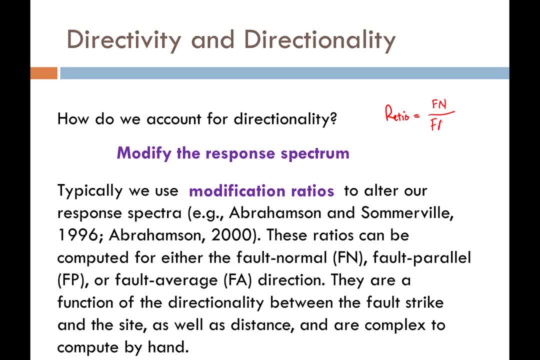 maybe fault normal, divided by the average value of considering all orientations, so the average of all the different directionalities. So all I need to do, then, is multiply the average ground motion by whatever this ratio is, and voila, I get the increased ground motion. 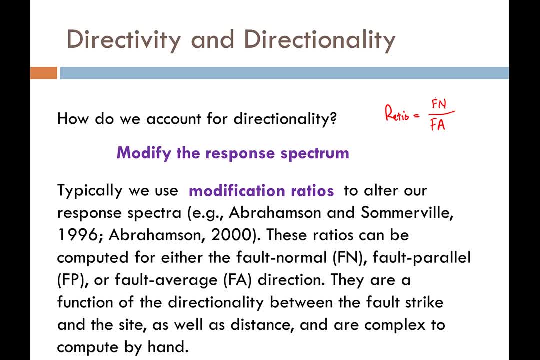 according to the maximum directionality. So this idea was originally proposed in the late 90s, early 2000s by legends Norm Abramson, Paul Somerville- Later Abramson modified it And all of these models that did this. 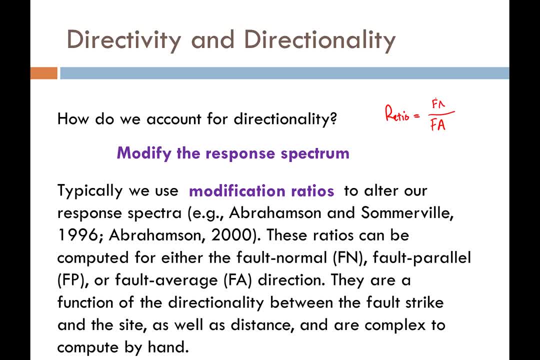 they were all based on two orientations, either normal to the rupturing fault or parallel to the rupturing fault, And so it was widely believed that the fault normal orientation gave the strongest ground motions and fault parallel orientation gave the weakest motions. Now, these models are not easy to compute by hand. 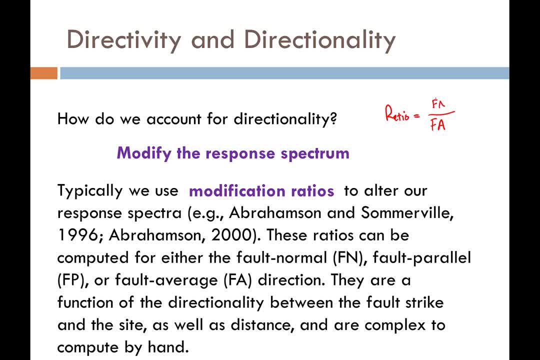 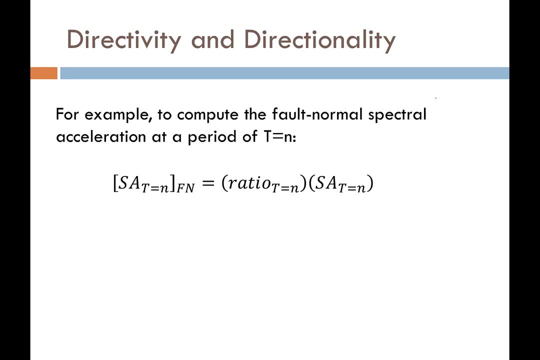 and so typically they were computed by a computer that was also doing the seismic hazard analysis, and it was just added into the seismic hazard analysis. So if I wanted then to compute the fault- normal acceleration instead of just the average, what I would do is I would take my ratio. 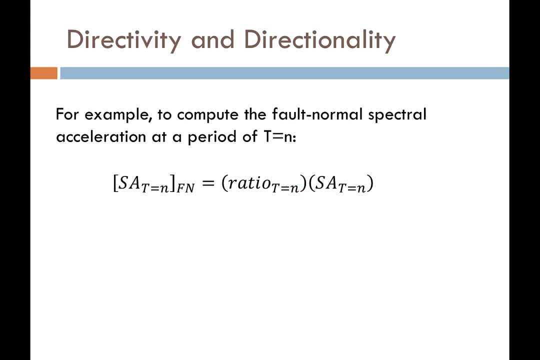 that I would compute from whatever these models were and I would just multiply it by the spectral acceleration value at the appropriate period. So again, these ratios are a function of the period, so it's not just one constant number. Different periods have different ratios. 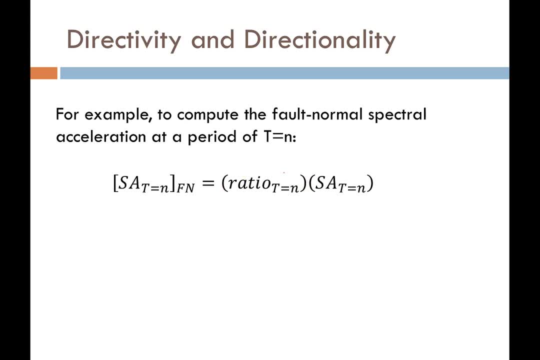 or different multipliers by them, And bear in mind that these ratios really only apply to periods that are greater than half a second. Anything that is less than half a second, the ratio is always equal to one, So it doesn't really affect it. 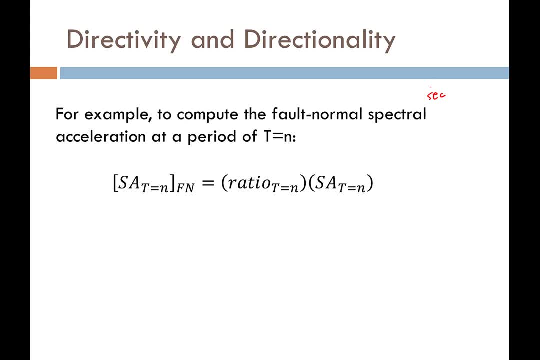 But for these longer period stuff, directionality makes a big deal, at least in the response spectrum. So in my experience what I've typically seen is that that fault normal ratio from these models ranges anywhere from 1 to 1.5.. 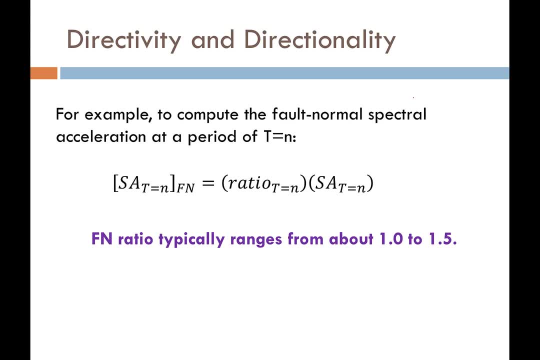 So think about that With 1.5, you're increasing your ground motions by 50% just due to the maximum orientation of those ground motions, And so that's a big deal For the fault parallel. the ratio ranges from anywhere from 1 to 0.85.. 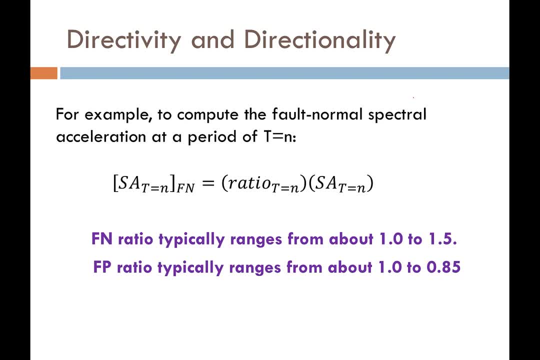 So we're potentially reducing the response spectrum up to 15%. Now I cited these Abramson and Somerville models, and when we use the NGA West models, however, nobody really uses those Abramson and Somerville models anymore. They're not really appropriate. 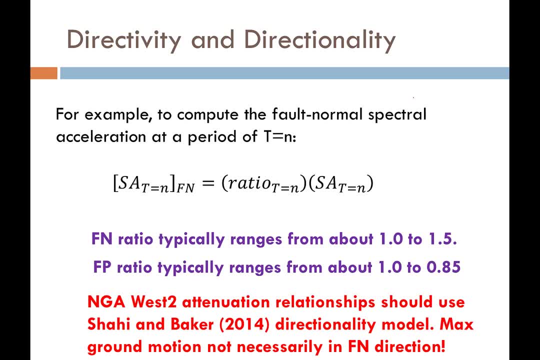 Instead, everyone uses a model developed by Shahi and Baker in 2014,, and it will give you the maximum directionality or the maximum rotated ground motions. The interesting thing, though, that Baker pointed out is that, in their statistical analysis, 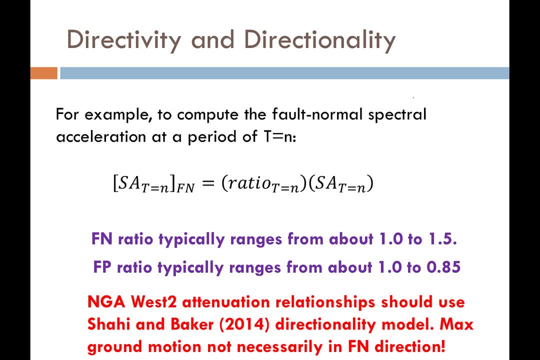 that maximum rotated ground motion does not always align with the fault normal orientation. Sometimes it's a little bit off fault normal and so this kind of long-standing belief that fault normal is the maximum direction of ground motions. they've basically shown that that's not really true. 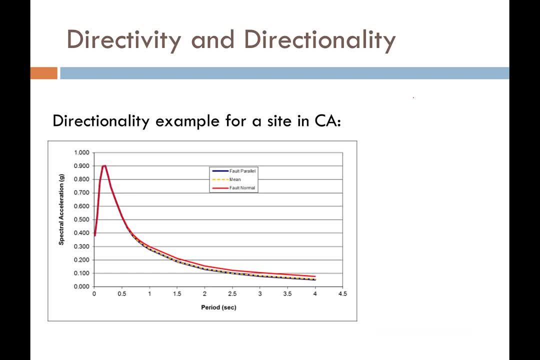 So here's a figure that I pulled from an actual analysis that I did as a consultant years ago. I know it's not like grandiose, but you can see that at a period of half a second these response spectra split. 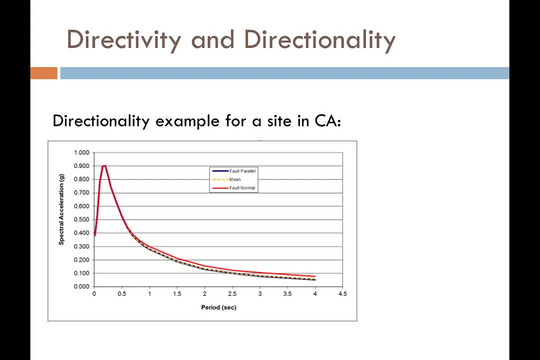 and I've got a fault normal response spectrum, I've got a fault- parallel response spectrum, and then I've got the mean or the average, And so you can see that the fault normal response spectrum is approximately 25% larger than the mean response spectrum. 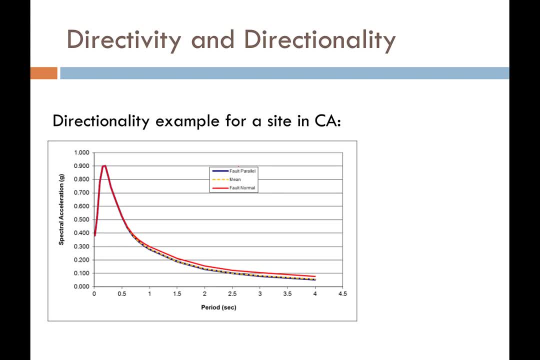 and then the fault parallel response spectrum is maybe in this case about 5% smaller than the mean response spectrum. So it's something that we want to take into account again when we are trying to be as accurate as possible as predicting the ground motions. 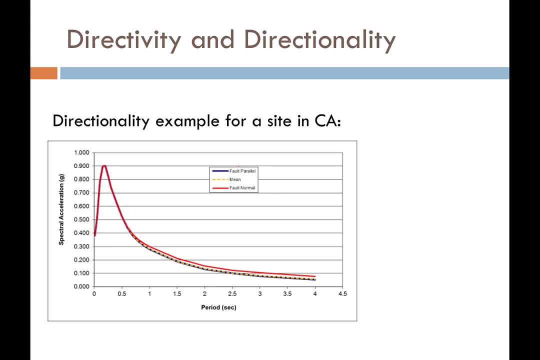 that our site could experience Accounting for directionality and directivity are really important, these near-source effects, And again remember that these directivity and directionality effects, they're really only going to affect periods in your response spectrum that are greater than half a second. 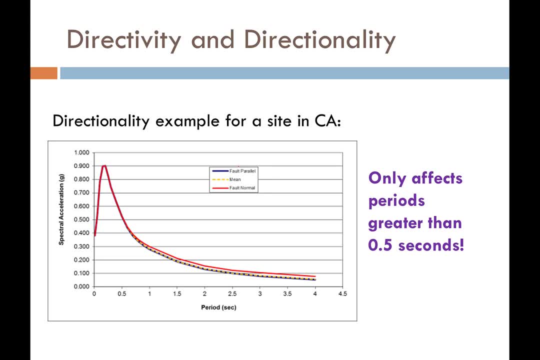 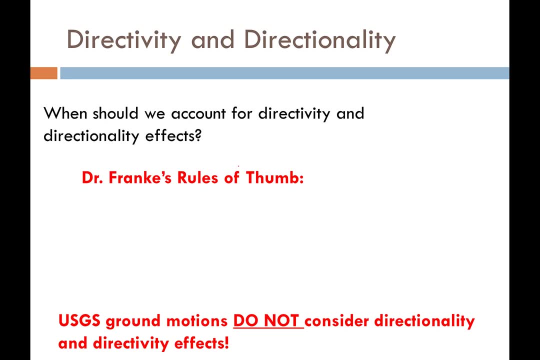 These low-period, high-frequency portions of the response spectrum. they don't really affect those. So back to my rules of thumb. when should we account for near-source effects, directivity and directionality? Well, here are my rules of thumb. 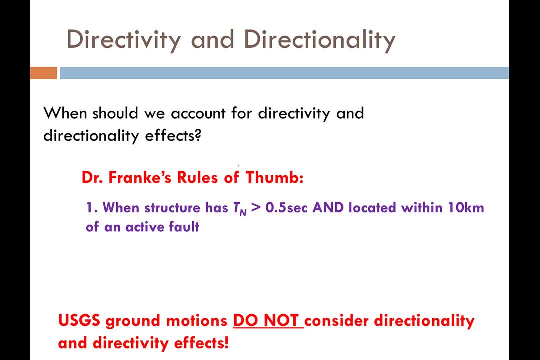 Number one is when your structure has a natural period of vibration larger than half a second and you're located within 10 kilometers of an active fault, Because- remember near-source effects- they have nothing to do with the soil type, They have everything to do with your proximity. 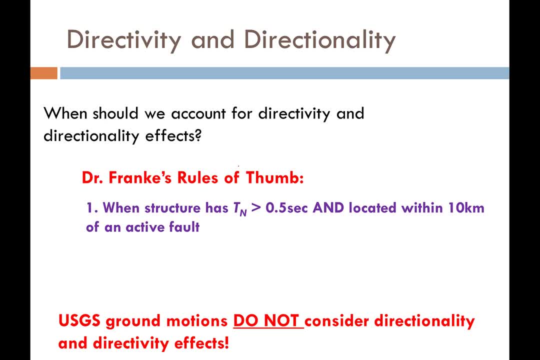 to the rupturing fault and that's it. It doesn't matter if you're on gravel, sand, clay- the soil is inconsequential. It's your location relative to the rupturing fault that affects near-source effects. So that's the first one. 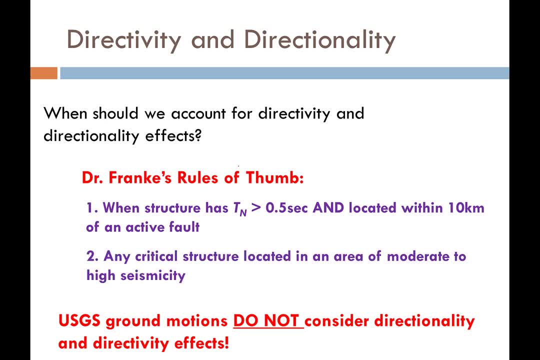 And the second would be any critical structure located in an area of moderate to high seismicity, And the reason for that is we don't necessarily know where the faults are, And if you're in an area of moderate to high seismicity, the chances are there's probably a fault. 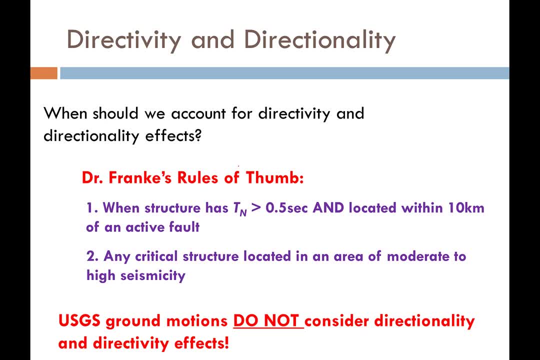 beneath your feet anyway, And if that fault goes, you could potentially experience these near-source effects yourself. Now it may surprise a lot of people to learn that the ground motions that are computed by the US Geological Survey and provided for free to the public. 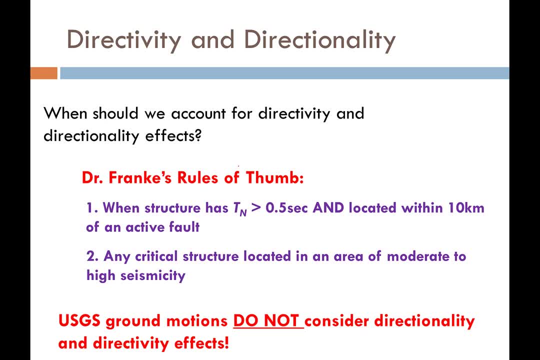 for use in, like building code. they do not consider directionality and directivity effects. They don't consider near-source effects. I don't understand why They just don't. And so that makes it challenging because new revisions of the code 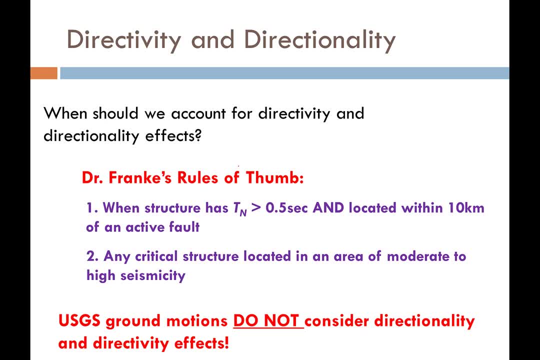 the IDC 2018,, for example, requires that a ground motion hazard analysis accounts for near-source effects, And so we're kind of in this uncomfortable position right now, as the code is getting learned and engineers are getting comfortable with it, And I'll talk more about that. 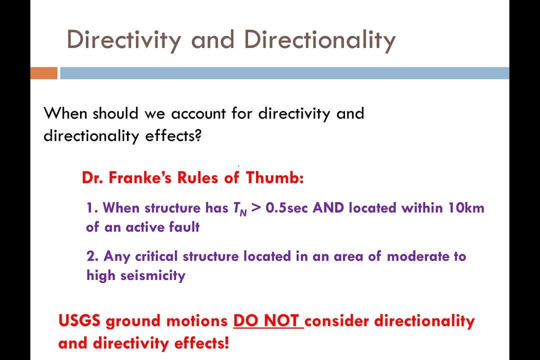 in the next lecture, but it's a tricky spot right now and we're all still trying to figure it out. But just be aware that if you want to consider near-source effects- and you should if you're trying to comply with code- 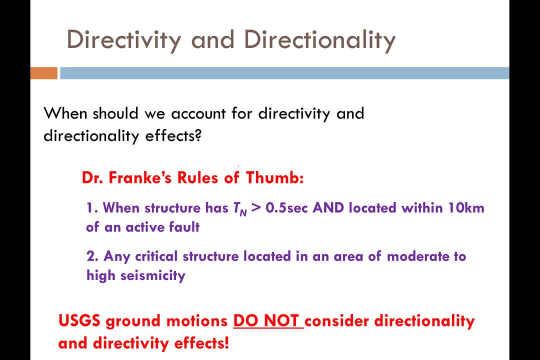 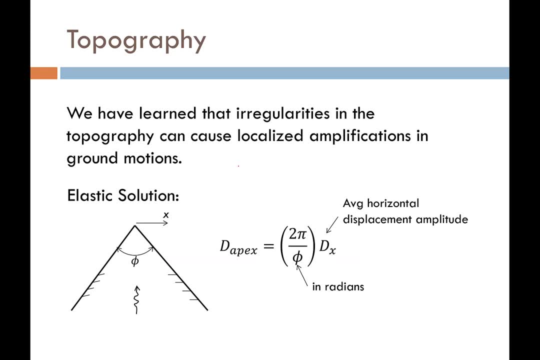 you're going to have to add those effects into your response spectra yourself. Okay, Let's talk about the third local site effect, and this is topographic effects. Now, topographic effects, it's kind of intuitive if you think about it. 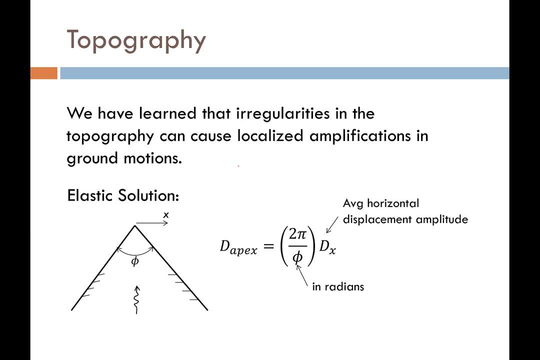 So if you go take a like a stick or a reed and you hold it up and you kind of whip it back and forth, you can whip and crack the end of that stick or that reed And so there's a whipping effect. 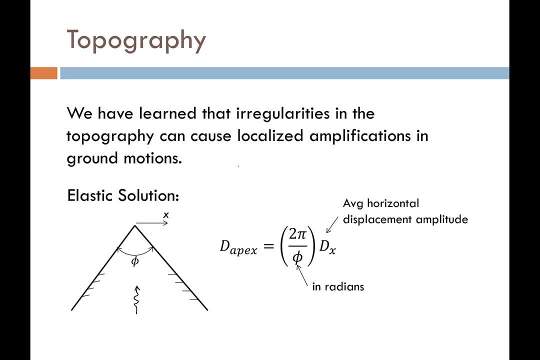 whenever you have a protruding topography, And the same is true when we just have the surface of the Earth. So, as we see down here in my bottom left, if I have a hill or a mountain or a steep slope and I'm located up here at the peak, 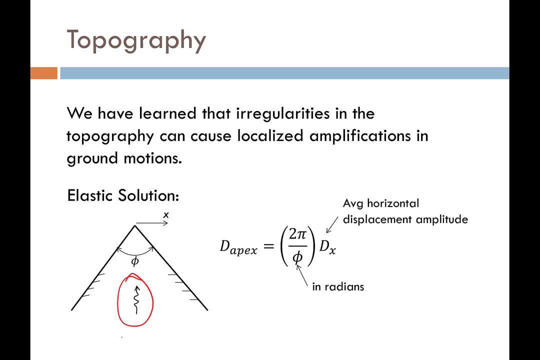 and I have an earthquake, ground motion come into and shake the bottom of that thing, so the whole thing starts moving. the top of this peak is going to get whipped, And so the displacement that I experience at the top versus the displacement that I might experience at the bottom. 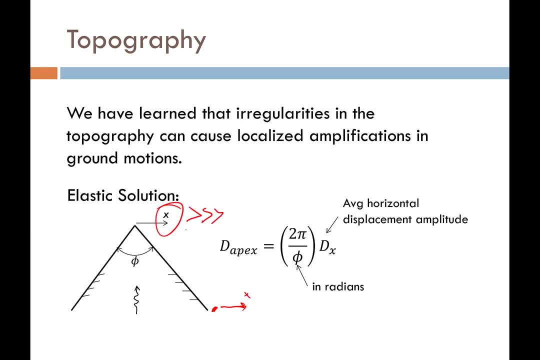 this displacement is much greater than this displacement down here because of the whipping effect that occurs. And so you know, we know this just intuitively, but mathematically we can try to explain it And really what happens is, if you think about, you know. 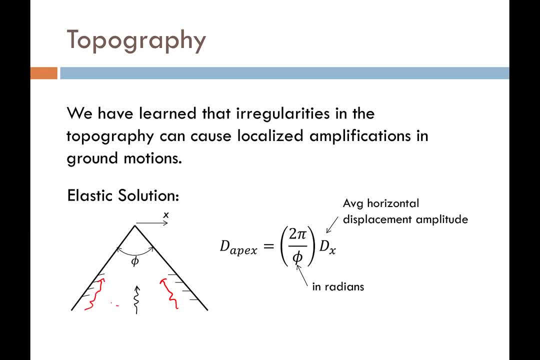 there's waves over here, and there's waves over here, and there's waves over here. all of those waves just converge, converge, converge into a single point, And what we end up having, mathematically, is an infinitely large amount of energy focused on that single point. 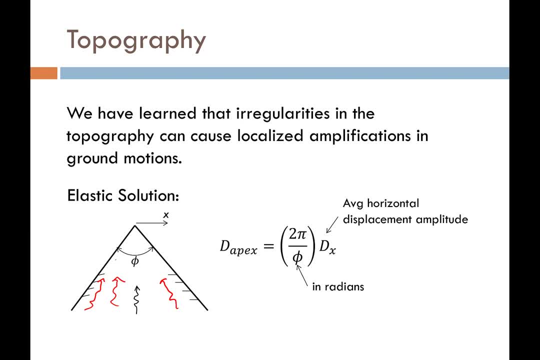 right on the peak, And so we end up getting some pretty large displacements at the apex of that peak. So interestingly though, the math rarely matches what actually happens in the field, and that's because there's other effects in play, like 3D effects and damping. 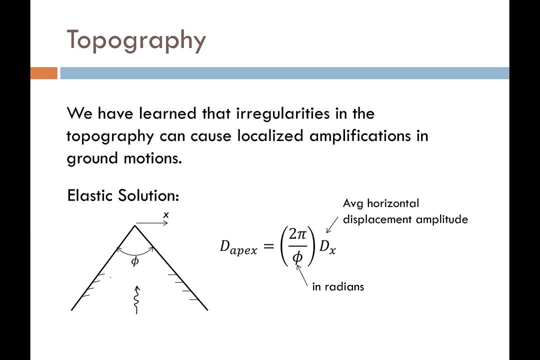 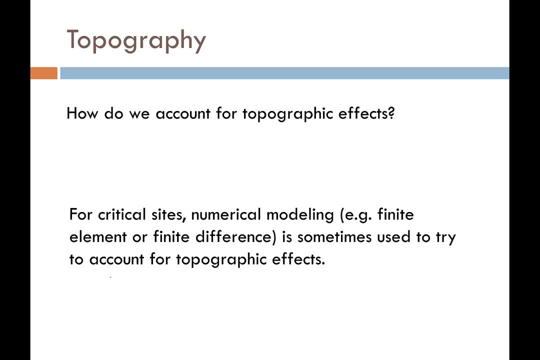 and attenuation of the energy and things like that, But at least they get us in the ballpark. So if we want to account for these topographic effects, how do we do it? Well, the truth is we usually don't. We usually don't just because 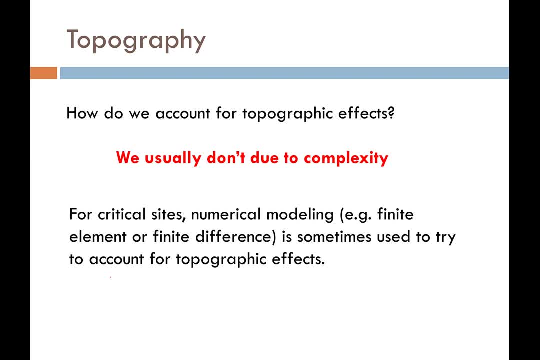 it's hard to do it accurately, And to date, the only way to get even close is you need to run a beefy numerical simulation, And for most projects that's well outside the scope of what we're trying to accomplish, And so usually we don't. 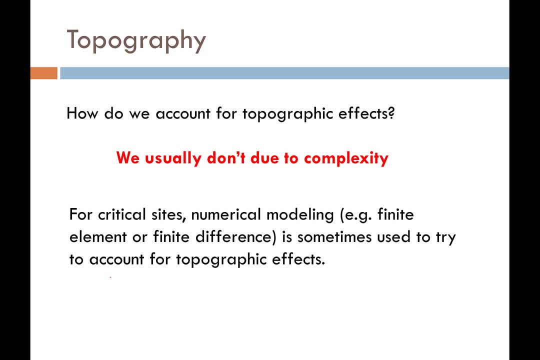 We don't account for it, Should we? Well, in my experience in the reconnaissance I've performed around the world in the last few years, I've definitely noticed a pattern that the largest damage often is concentrated around the slopes and on the tops of the slopes. 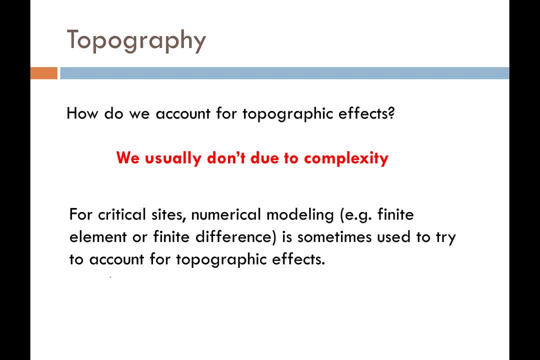 and the peaks. You know, human beings are interesting creatures. We like to live up high, We like to look out and have great views and look down on all the people that we perceive to be less than us. And so everybody likes to build. 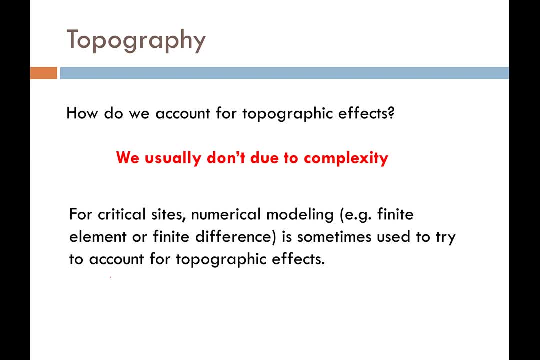 on the mountains or on the benches way up high, And what we've learned from experience when it comes to earthquakes is those are often the places that get shaken the hardest. So yeah, that may not satisfy you to say that we don't consider these things typically. 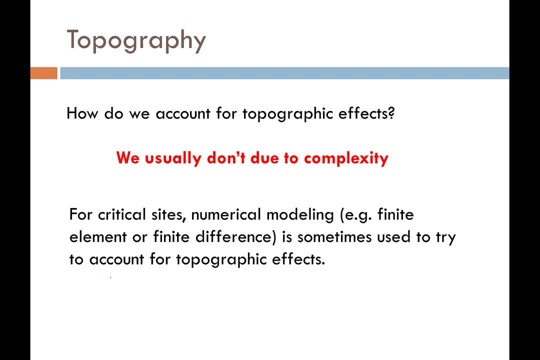 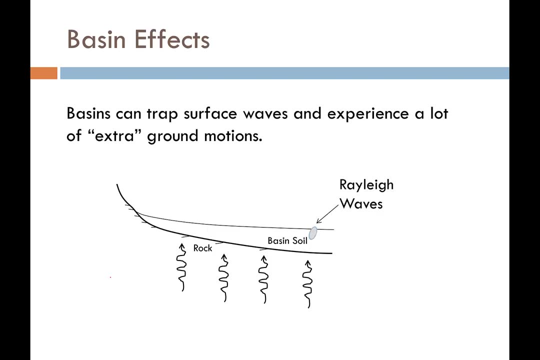 Maybe someday we will, But currently we just we know that this is a very common factor, We kind of account for it just in our judgment, but we don't really assign any numbers to it. Okay, the last effect that I'm going to talk about. 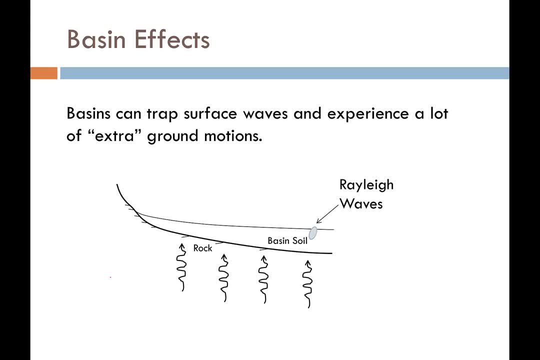 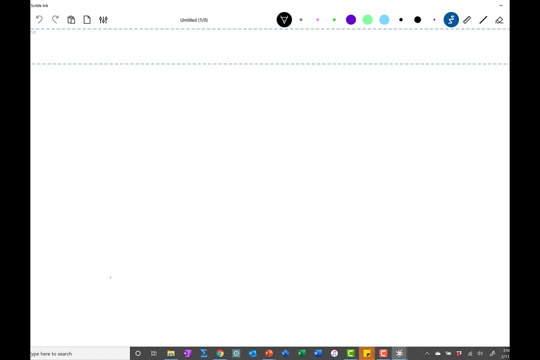 is called basin effects, And this is a big one. So what is a basin? A basin is basically a valley, right? So if I take a cross-section, for instance, of Utah Valley where Brigham Young University is, I may have the Wasatch Mountains. 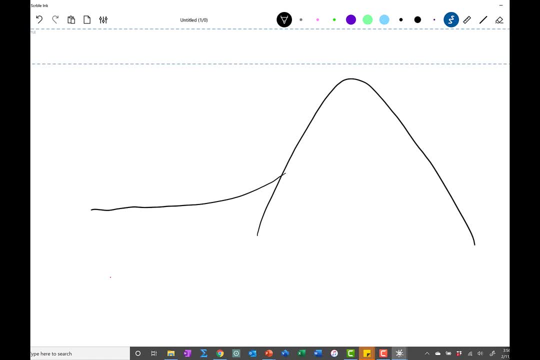 off to the east. Then I have the valley, I even have the Utah Lake right here, And then on the other side I've got the Ochre Mountains. And you know, these bedrock come down and at some point they intersect. 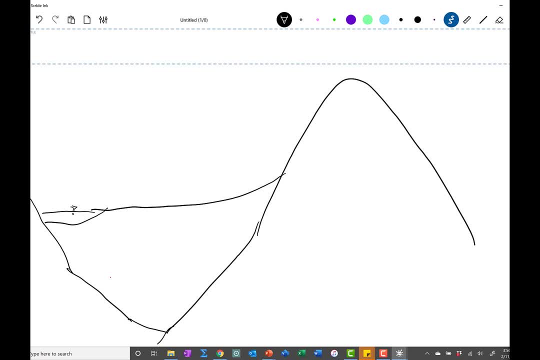 And so we have this valley, this sediment-filled valley, And this right here, my friends, is what a basin looks like. Think of it like a giant bell or a bowl, meaning that energy can come in and come to this other side and bounce back and forth. 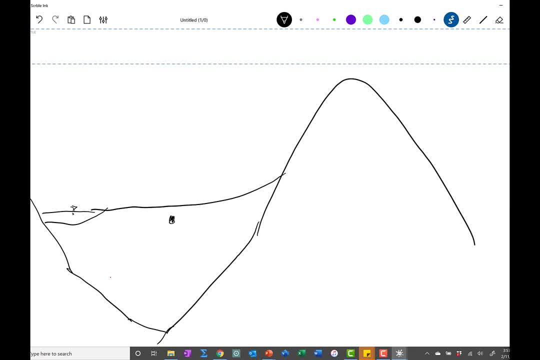 Or if, once energy gets inside of the soil and it starts going out in all directions, it hits the rock and it reflects, and it just vibrates and reflects back and forth, kind of like the ringing of a bell. And so that's why oftentimes basin effects 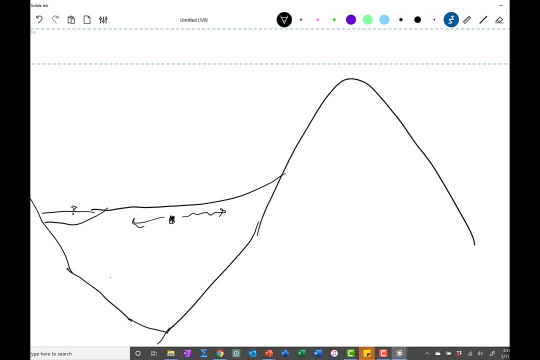 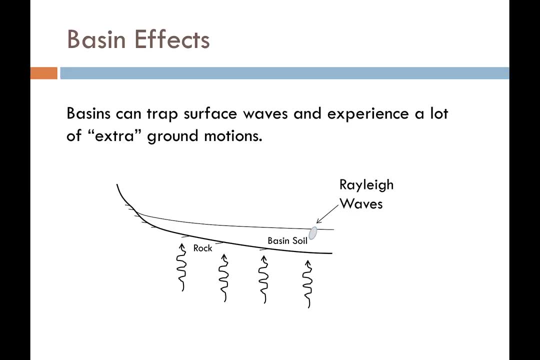 are likened to the ringing of a bell And a lot of the same physics apply, but I'm going to talk about one particular aspect of basin effects. So you get, of course, the reflection and the echoing of these ground motion waves, as the waves reflect and bounce back and forth. 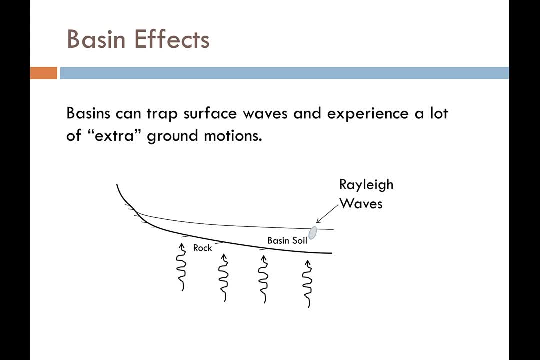 off these walls. But there's another effect that is associated with basin effects And it deals with the surface waves, particularly the Rayleigh waves that are traveling through the soil. So I've made this little animation here. Here's Rayleigh waves from an earthquake. 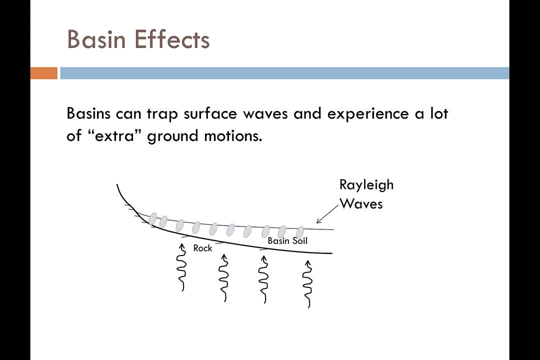 And they're traveling through the soil and they're in all directions and these waves are heading And eventually the soil starts to get thinner and thinner and thinner as we approach the rim of the basin and we get to the rock, And as the soil gets thinner and thinner and thinner. 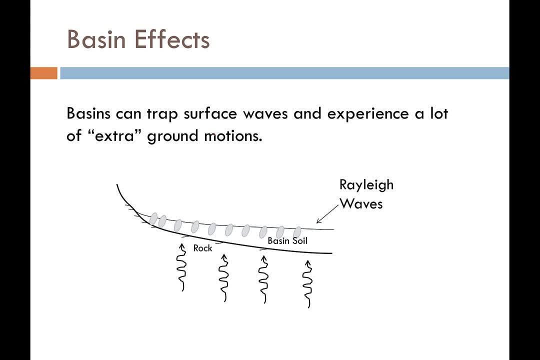 these waves. they want to maintain the same height, but the soil gets thinner. So notice what happens as we get close to this rim. It looks like the waves start to kind of rise out of the soil because they're trying to maintain the exact same height. 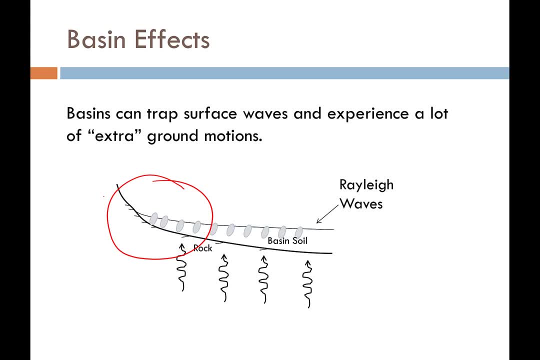 the exact same amplitude, And so we get an amplification right at the rim of our basin, And that amplification of the waves can be quite significant, And so, again, this would be akin to building near or on the benches of the basins. 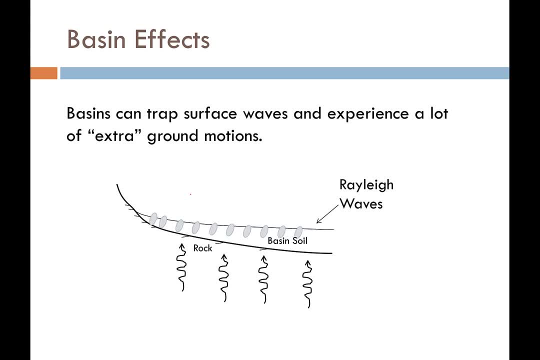 where in Utah everybody wants to live, And so those homes are probably going to get larger ground motions than homes that may be out here in the middle of the valley where the basin is deeper. But those homes down there will probably have other problems like soil liquefaction. 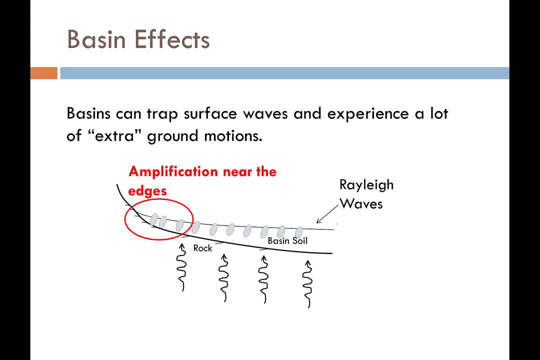 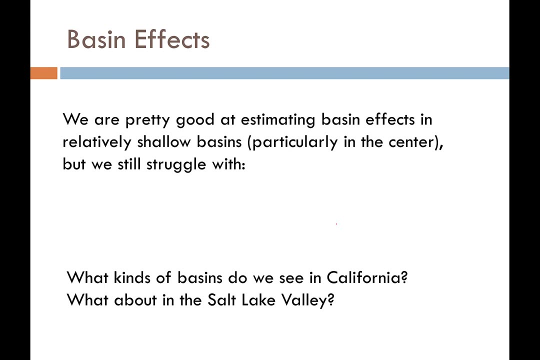 to worry about, But right here, this amplification near the edges of that basin. those are what we want to focus on here for these basin effects. So numerically we're pretty good at estimating these basin effects. We can capture them pretty well.